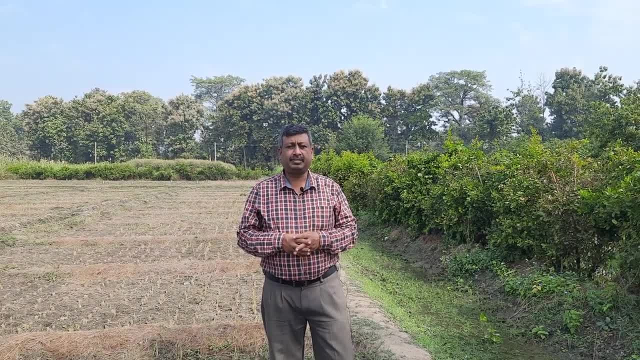 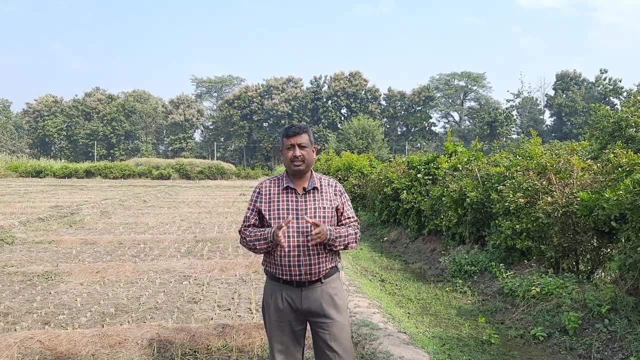 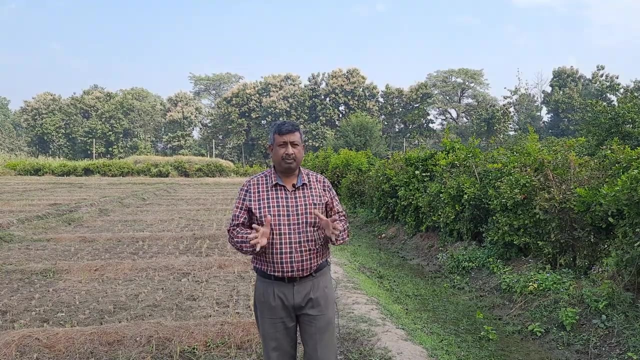 availability is hampered and ultimately yield is low. so for if this type problem is there, we should go for reclamation. but before reclamation we should check what, what is the soil ph and how this soil ph affect the nutrient availability. so in today lecture we will discuss this soil ph. 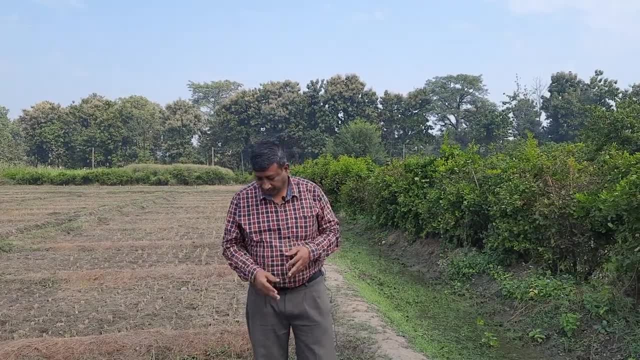 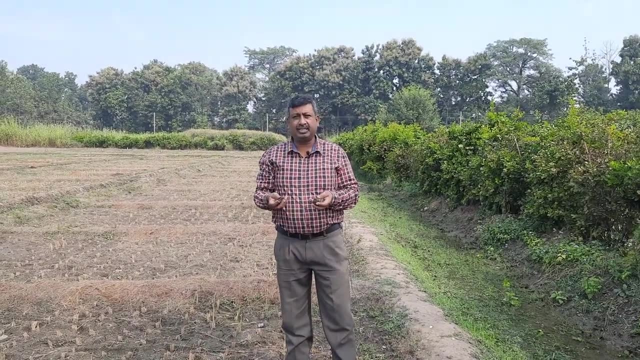 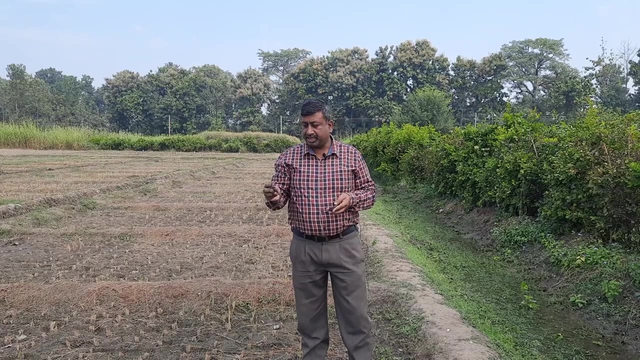 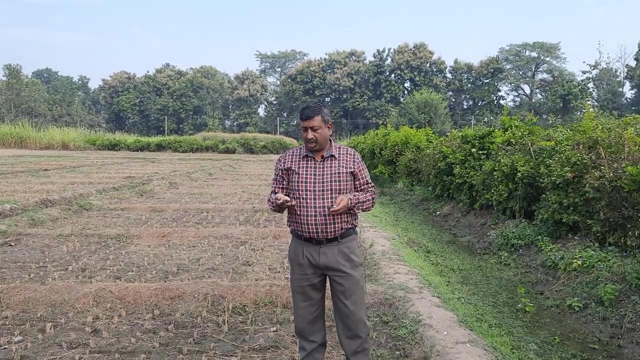 how affect nutrient ability to plant and if we see, we can see this soil and this soil. we can measure this soil ph in laboratory and this ph may be acidic, neutral or alkaline range, and the nutrient which are present in this soil may not be available if ph is not in optimum range. so how? 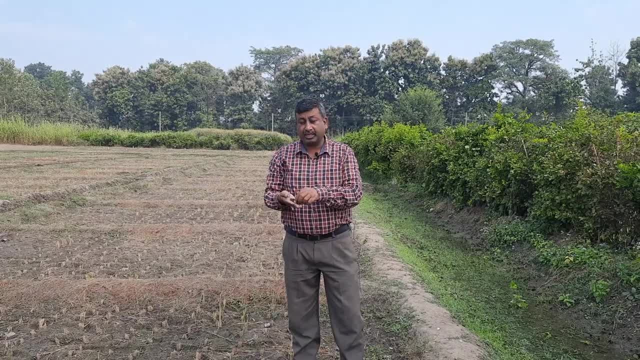 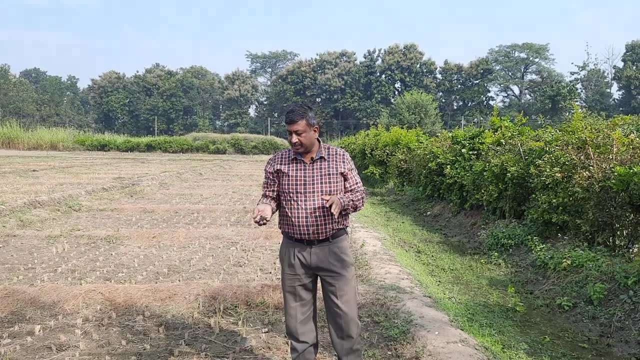 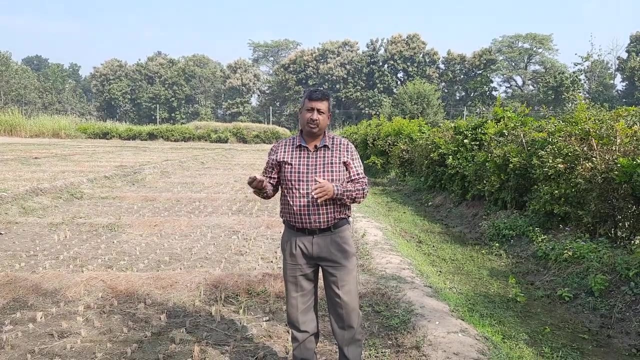 this nutrient, which are present in soil. they can. nutrient is present here, but because of change in ph these are not available to root. so this is very important aspect: that it contains nitrogen, phosphorus and potassium, but if this soil becomes acidic, then this nutrient will not be available to plant. if ph is very high, then also nutrient. 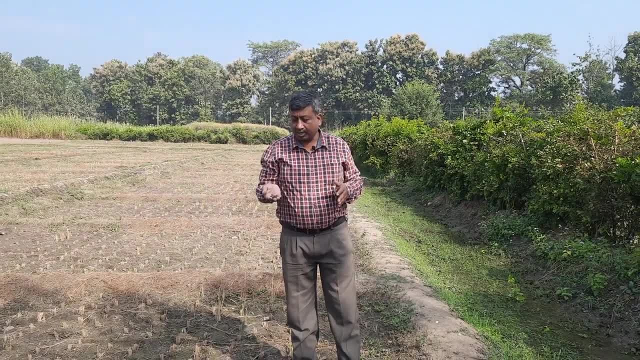 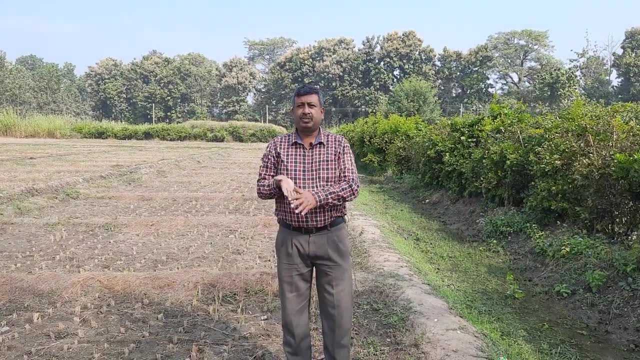 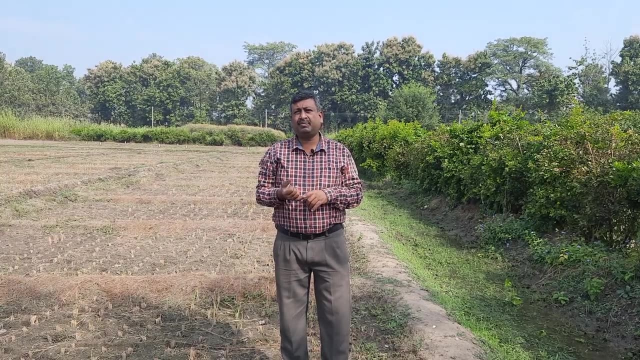 will not be available, despite the nutrient are present in soil. so what is the reason that nutrient is present in soil but it is not available to plant? so see nutrient availability is affected by ph by three means. number one: ph affect the nutrient solubility. so for any nutrient to be available to plant, it is 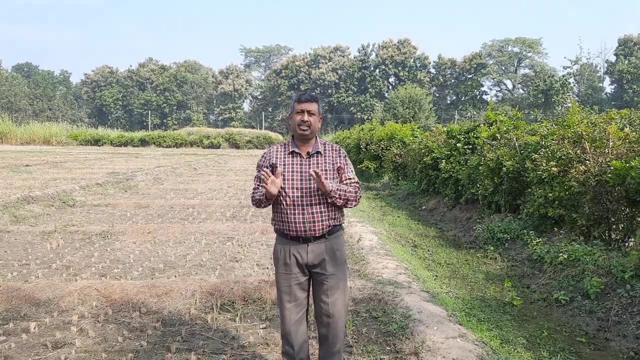 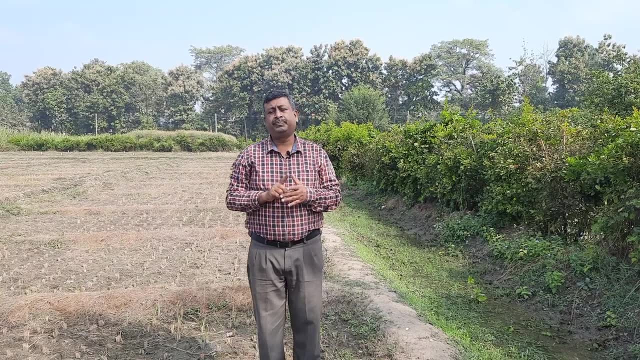 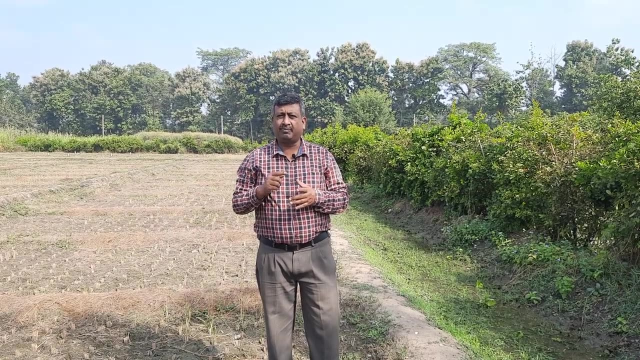 very important to be soluble, and ph affect nutrient solubility. this important aspect we should keep in mind. if nutrient is not soluble then it will not be available to plant. so number one factor is nutrient solubility is affected by soil ph. number two, microbial activity. microbes are involved in 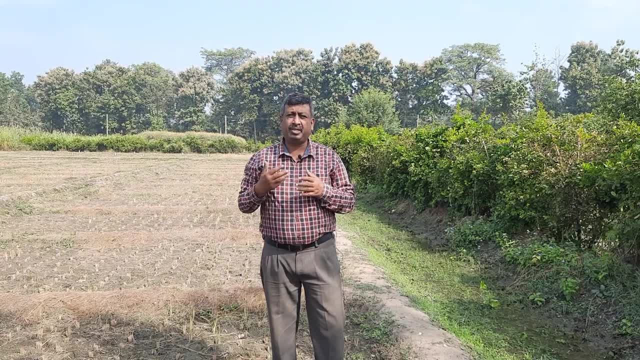 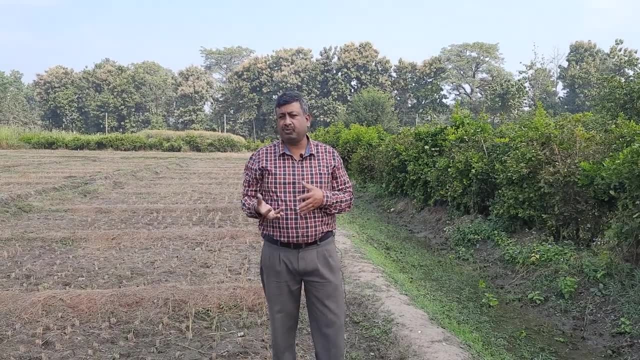 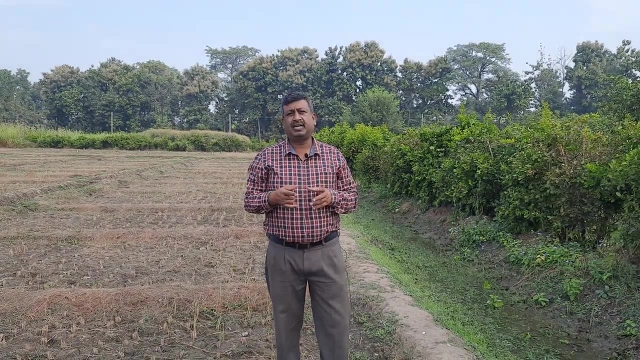 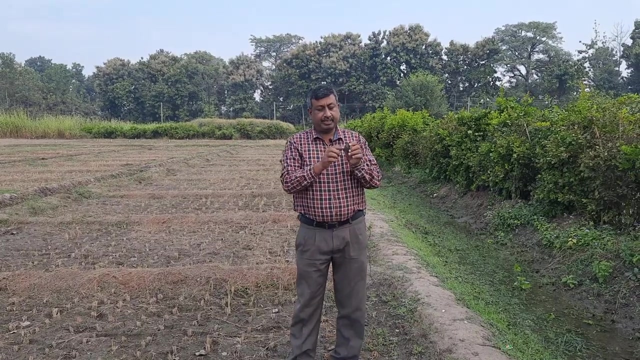 organometer: decomposition and mineralization. and by decomposition and mineralization nutrients are available to plant. so if microactivity is seized, then mineralization will not happen, and if mineralization does not happen, then nutrient will not be available to plant. and third factor is cation exchange capacity. so there is very important role of cation exchange. 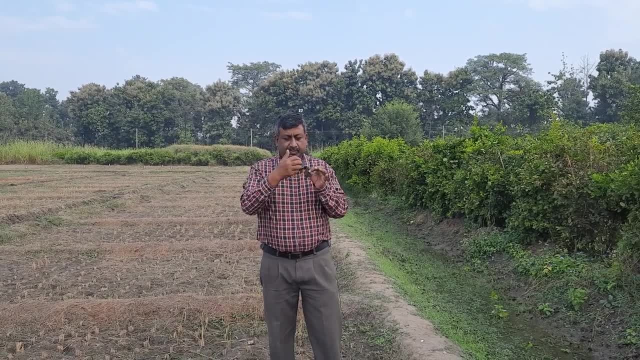 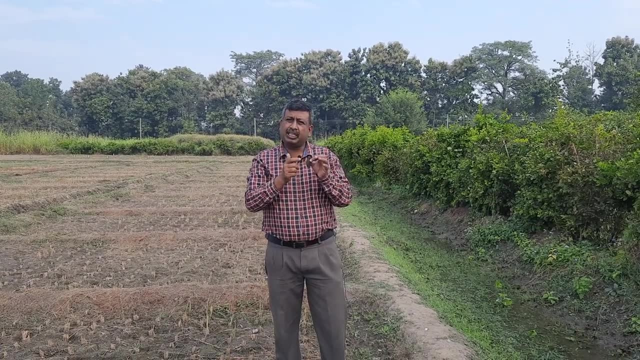 capacity. this is soil, it has nutrients and it are negative on clay particles. and what are cations above it? What is cation will come in the solution and where will the solution go? We will find this particle. This phenomenon continues that the soil solution cation comes on the clay particle and clay. 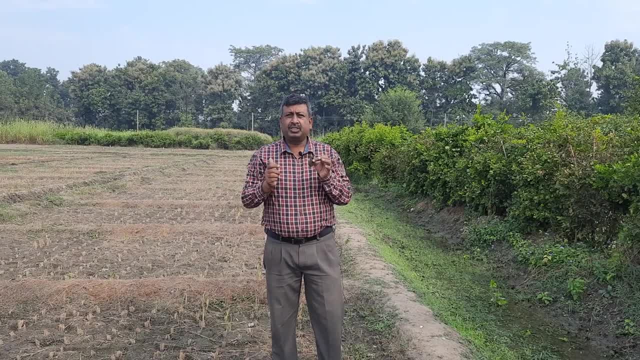 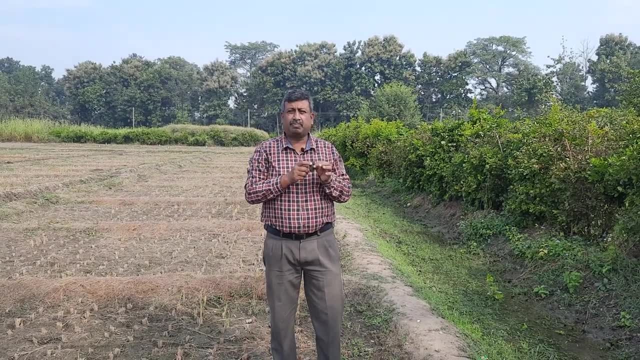 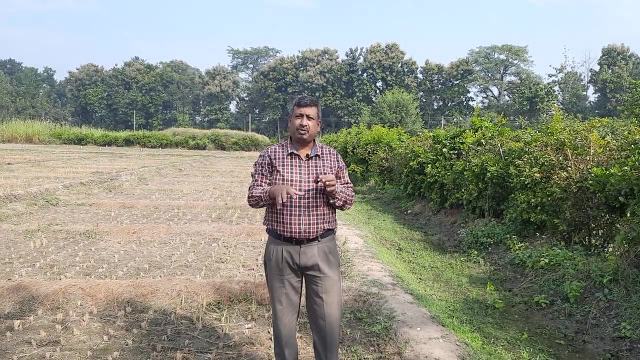 particle nutrients come into the soil solution And when it comes in the soil solution then the root absorbs it. The direct absorption of the root is very less than the soil particle. It is less than 1%. So 99% nutrients are absorbed by the root from soil solution. So if the 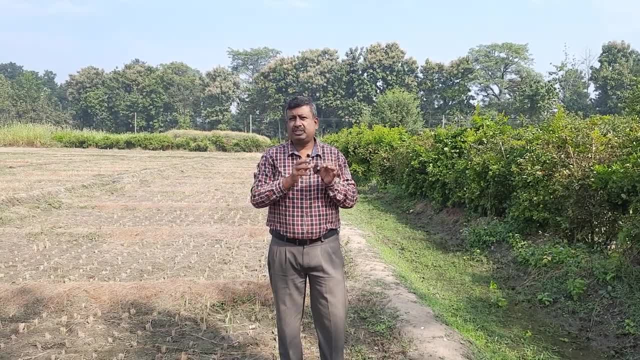 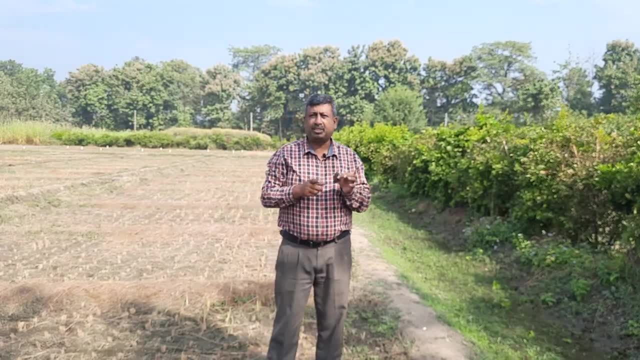 nutrient remains in the clay particle and cannot be absorbed by the soil solution, then it is not available for the plant. You have to understand this very well. Nutrient should be in soil solution, otherwise it will not be available to plant. How will it be available? 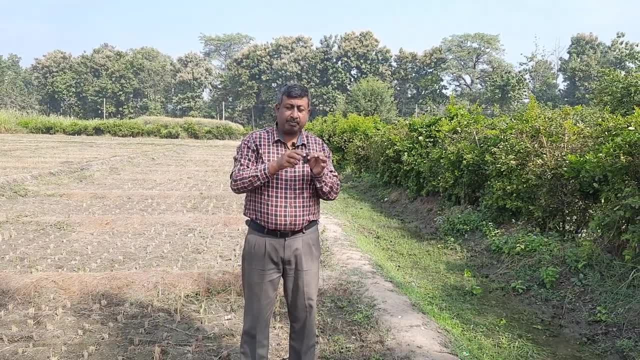 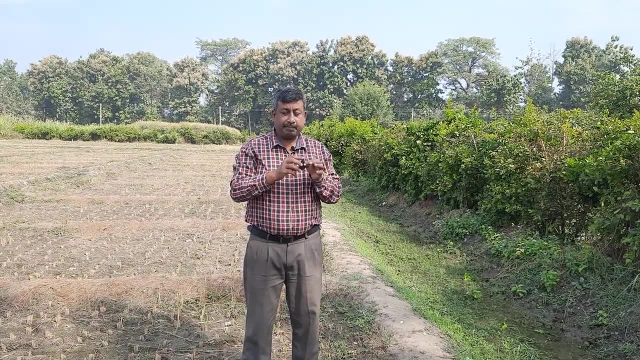 The nutrients which will be exchanged in the soil solution will be available in the clay particle and in the soil solution of the clay particle. This phenomenon is known as cation exchange And the capacity to do this is known as cation exchange capacity. So this phenomenon 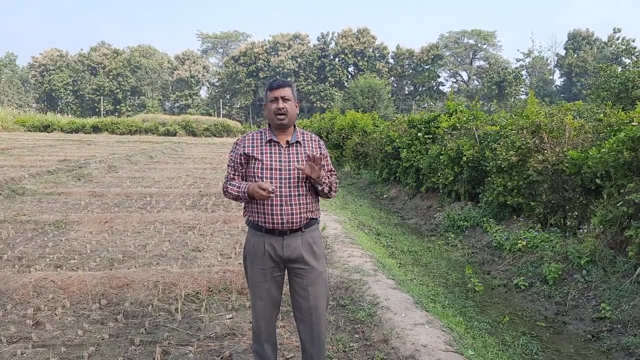 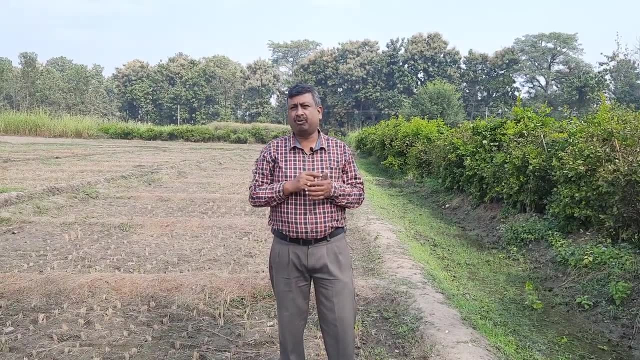 is also known as cation exchange capacity. This phenomenon is also known as cation exchange affected by soil pH. So now I have told you three factors how soil pH affect the nutrient ability. Number one is nutrient solubility. another factor is microbial activity and third, 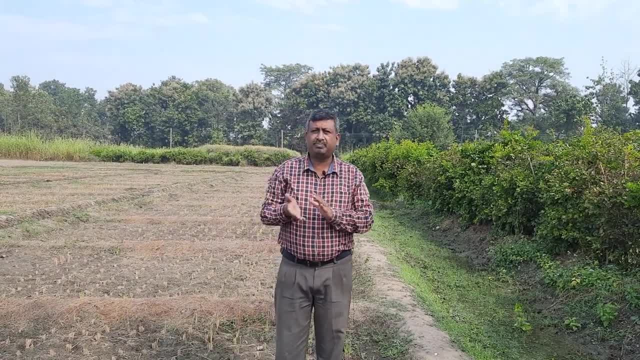 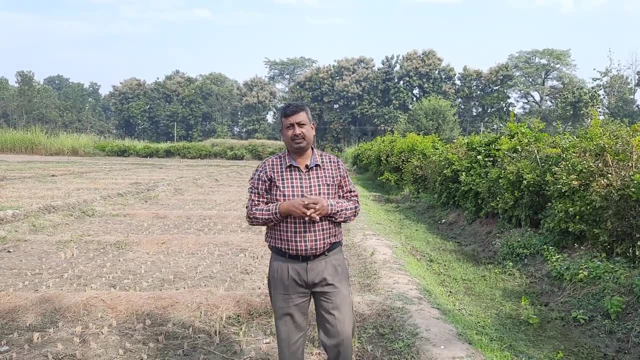 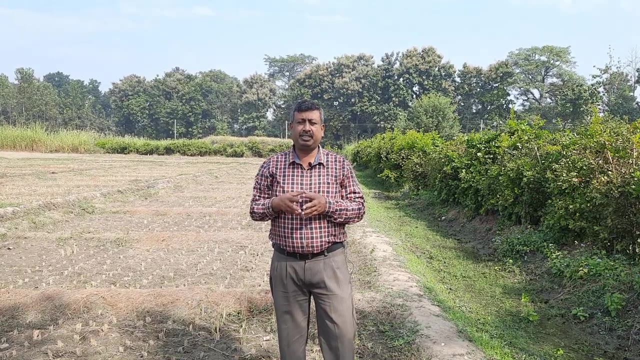 one is cation exchange capacity, So we will discuss this one by one. So, in case of nutrient solubility, if we look at essential nutrients, then number one. if we go from three, then nitrogen. and nitrogen is present in soil. in most of the nitrogen, 95 to 99 percent- is in. 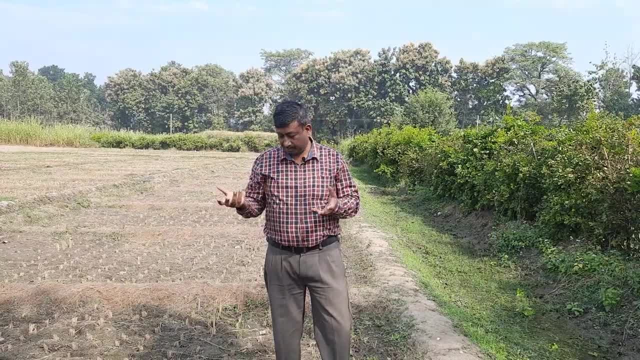 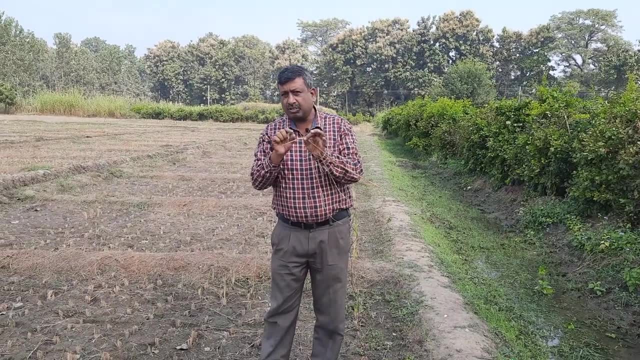 organic form and inorganic form is very less, And this organic form is present in residues. Nitrogen is present in plant residues And after the decomposition, whatever nutrient is present in it, it will come in soil solution And this decomposition is carried by bacteria. 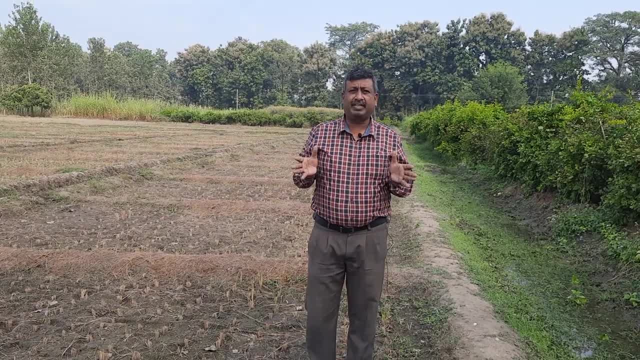 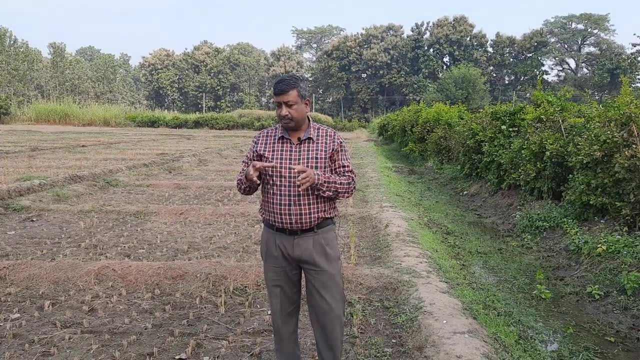 And whatever nitrate will be formed. there are so many bacteria, and important one are nitrosomonas and nitrovector. If this is not a bacteria, then it is a nutrient. So if it is not a nutrient, then what will happen? Decomposition will not be proper and its mineralization 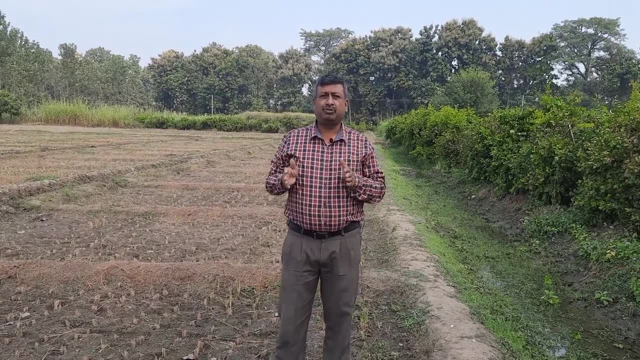 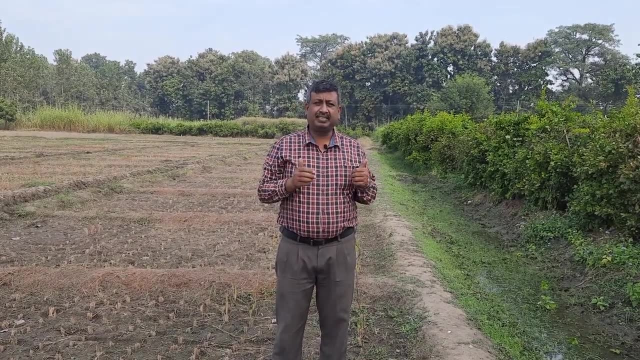 will not happen and then nitrogen will not be available to plant, And this nitrosomonas and nitrovector, particularly these two bacteria, perform better at neutral pH. So if soil pH is acidic, then bacteria activity will be very less and mineralization will be very. 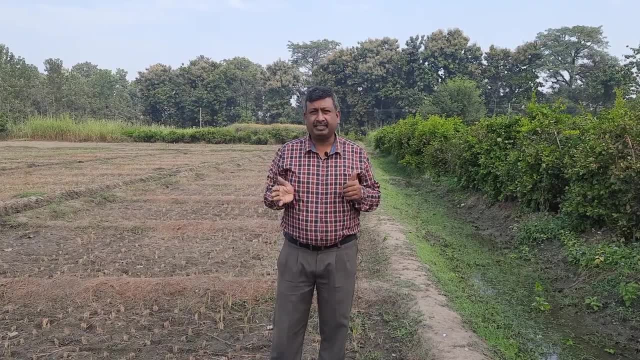 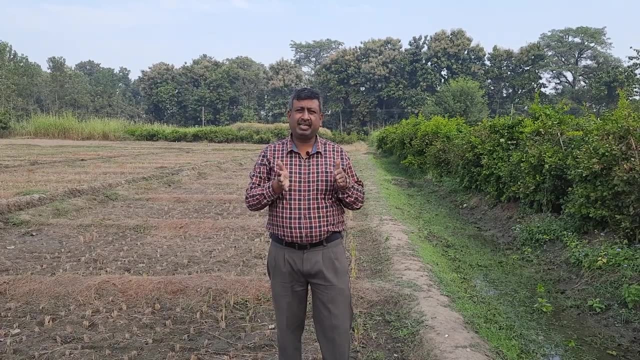 poor. That is why nitrogen ability will be very less. So in the case of nitrogen, it is very important to have neutral pH, Otherwise bacteria will not perform. And if we look at bacteria, if we talk about fungi, then fungi will not perform. So if we look at 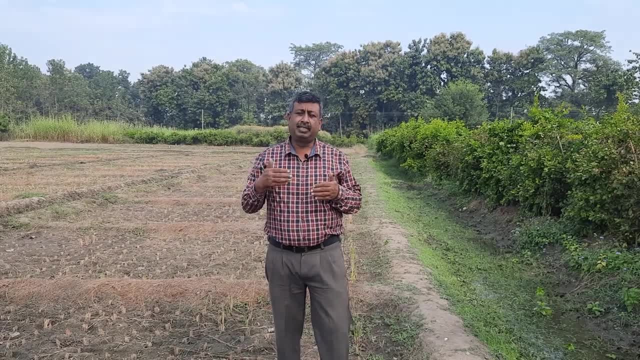 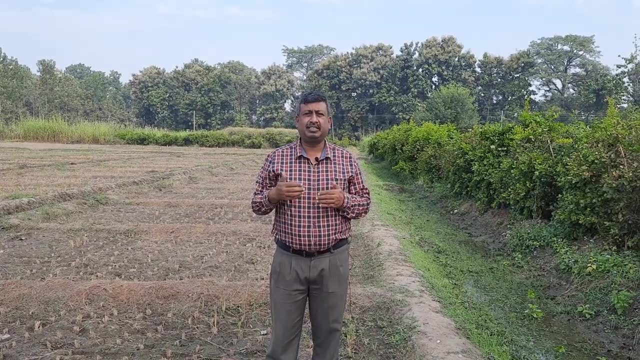 bacteria. then fungi are active at acidic pH and bacteria are active at neutral to alkaline pH. So the conversion of nitrogen from organic form to inorganic form, that is mediated by microbes, particularly by bacteria, And bacteria perform well at neutral pH. That is why nitrogen 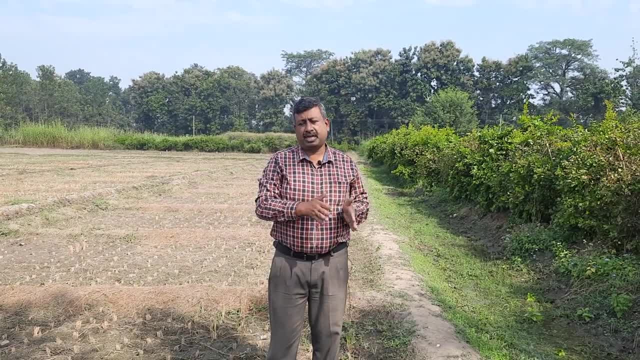 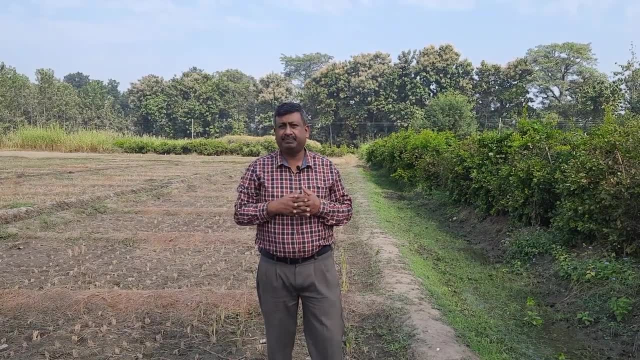 ability is maximum at neutral pH. So this was the case of nitrogen, And in the case of phosphorus, the mechanism is different. In phosphorus it is highly reactive. We know that phosphorus is very reactive- And in acidic soil it is highly reactive. So in the case 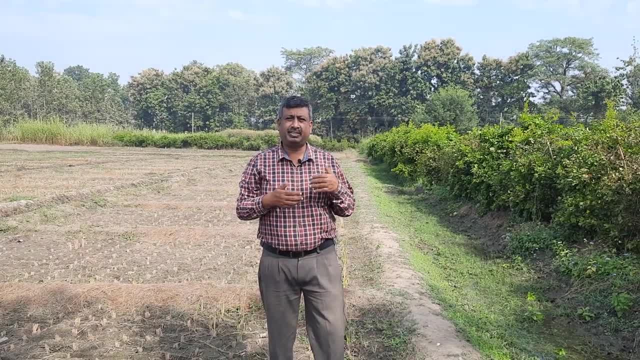 of nitrogen the mechanism is different. In phosphorus it is highly reactive. We know that phosphorus is highly reactive, So in the case of nitrogen it is highly reactive And in acidic soil phosphorus makes the complex, with the aluminum and iron particularly. 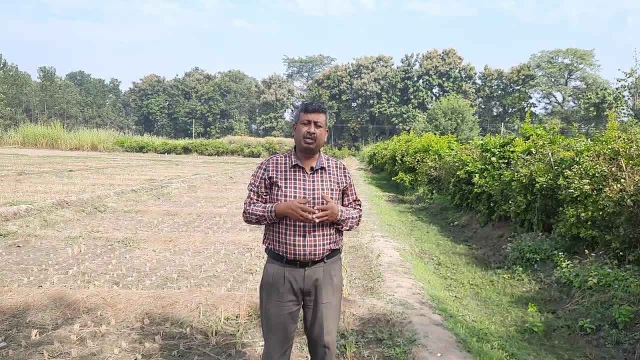 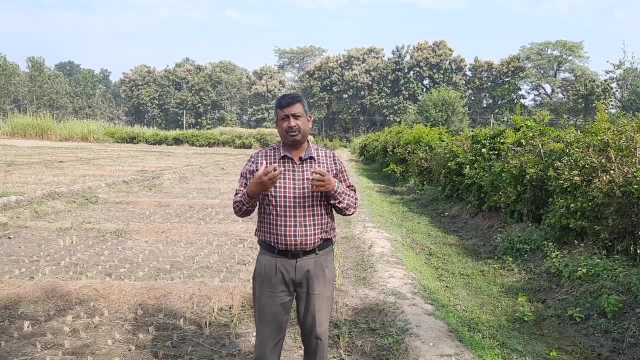 And this aluminum phosphate and iron phosphate are insoluble compounds And when it becomes insoluble the soil will remain in the solution. then the plant will not be available. I had told you earlier that for the absorption of a nutrient, its soluble form is very important. 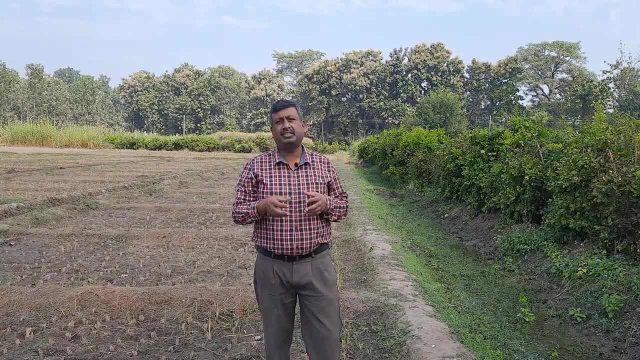 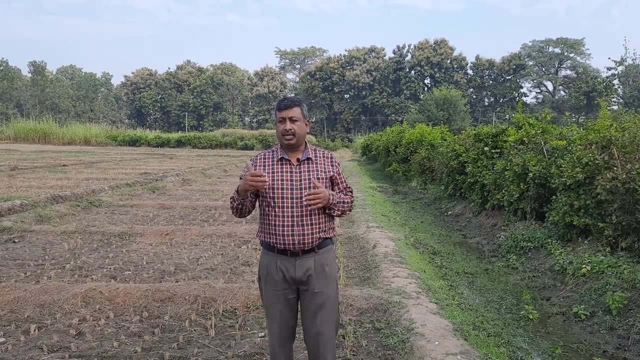 And this aluminum phosphate and iron phosphate are insoluble compounds. That is why phosphate or phosphorus availability is reduced. So this is the reason that phosphorus is not available in acidic soil. Now, on the other hand, if pH is high, more than 7, then calcium reacts with the phosphate And then again this calcium phosphate compounds. there are several: tricalcium phosphate, dicalcium, phosphate, apatite. Several calcium phosphates are there, and these are insoluble, or soluble is very less So that's why, at high pH, the 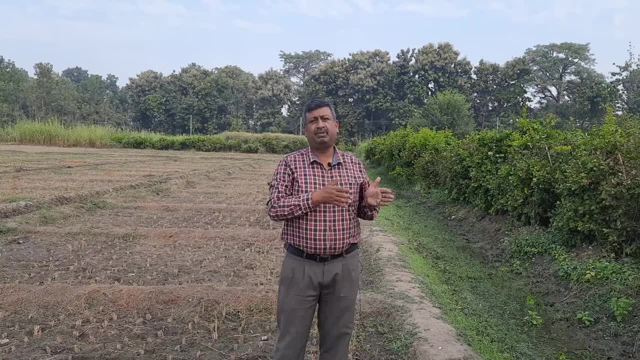 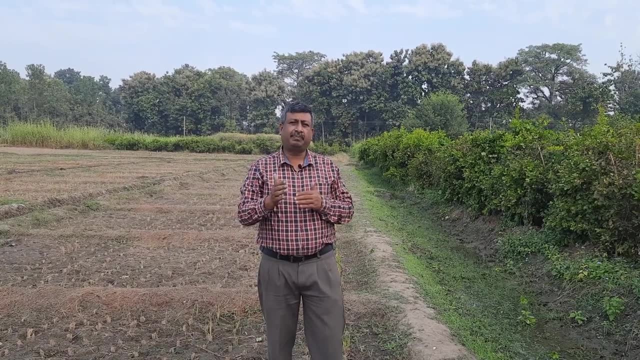 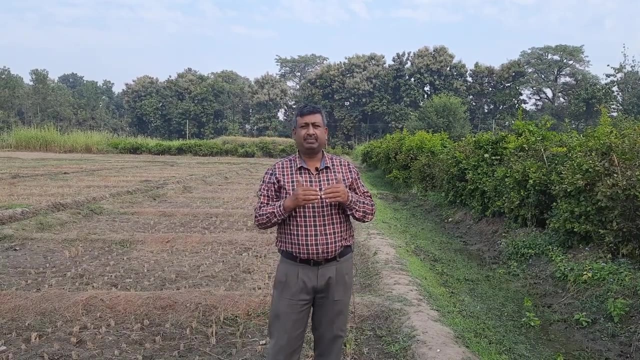 phosphorus, again, is not available. So this is the problem with the phosphorus. Neither it is available at the acidic range or NAR at alkaline range. So neutral pH range is almost 6.5.. Here on 6.5, the ability of the phosphorous is maximized, so we can say slightly acidic. 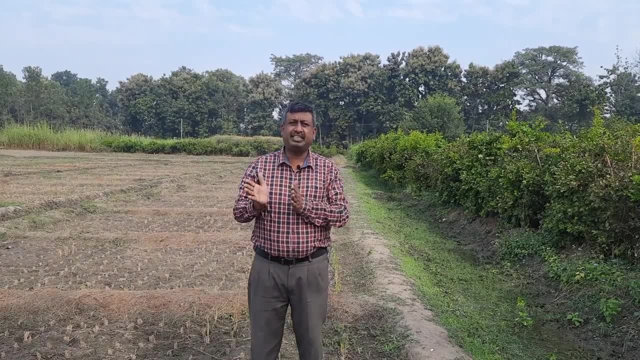 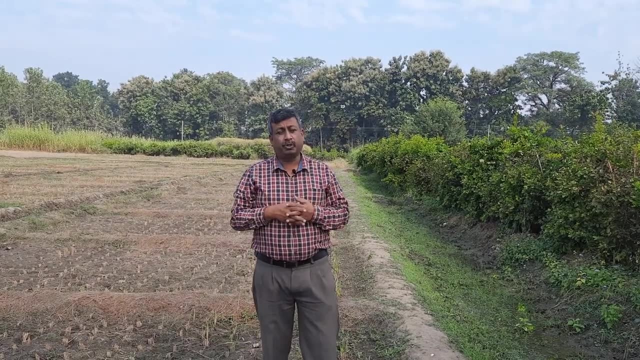 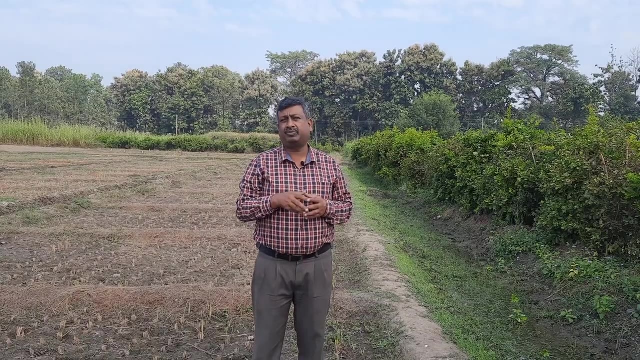 to neutral. So this will be a neutral pH range from 6.5 to 7.. So now again, phosphorus is available at neutral pH. Now the case of potassium and under acidic condition. potassium is monovalent cation and under acidic condition this potassium is replaced by hydrogen ion because under 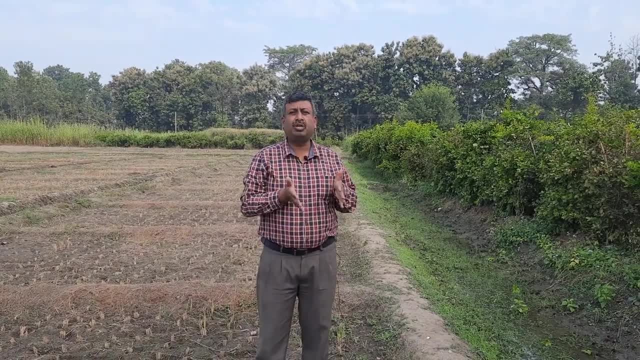 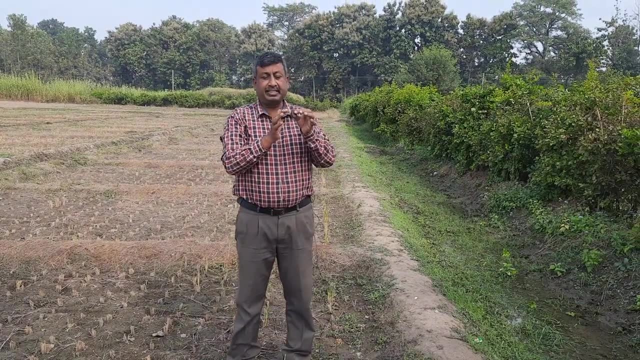 acidic condition, hydrogen ion dominate. So what will happen when acidic soil there will be a lot of hydrogen ion and what will this hydrogen ion do? That in the case of the potassium? in the case of the potassium, what will happen in acidic condition? that hydrogen ion will replace this potassium will replace a lot. 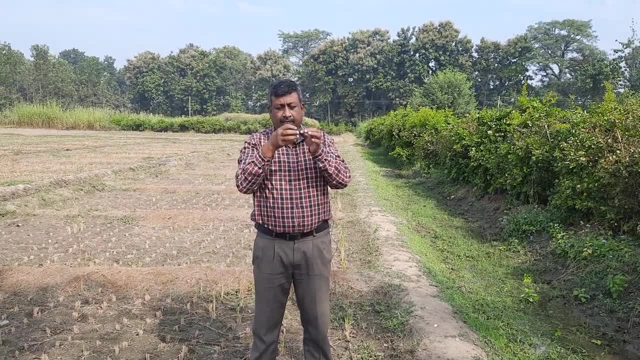 So where will all the potassium go? It will go in the solution. and what will happen in excess, when it comes a lot, it will leach. So under acidic condition there is a leaching of potassium. that's why ability is reduced. 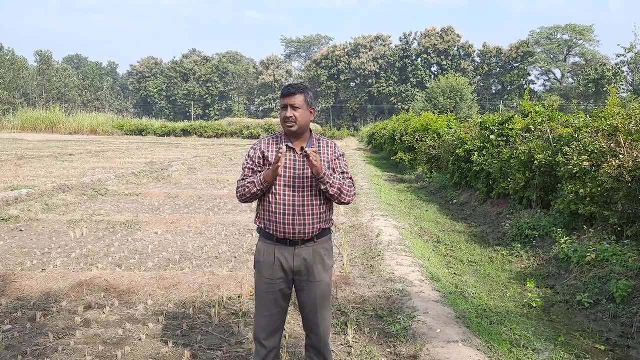 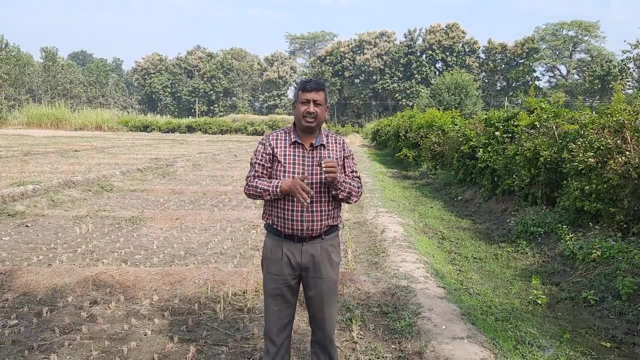 So it is also a problem to come to a lot of solutions. It should come to the solution. without coming to the solution, it will not be able to evaluate the nutrient plant, But if the excess is more than the requirement of the plant, then what will it do? it will. 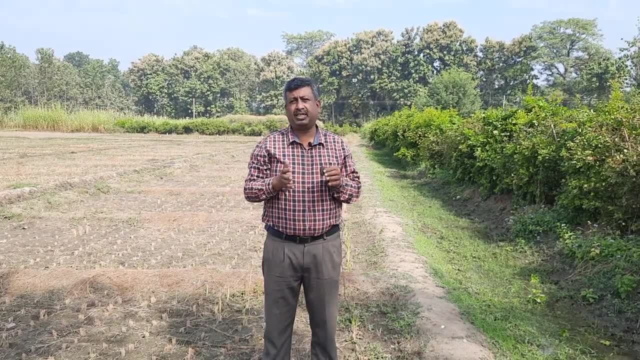 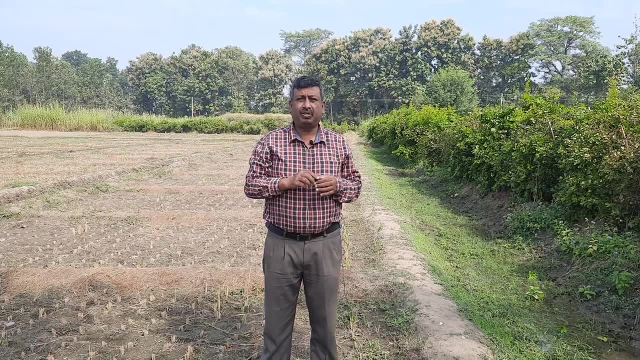 leach. So in acidic soil the problem is that potassium is replaced by hydrogen ion and there is a leaching. So there will be a leaching of potassium And if the soil pH is more than 7 and it is going in the alkaline range, then potassium 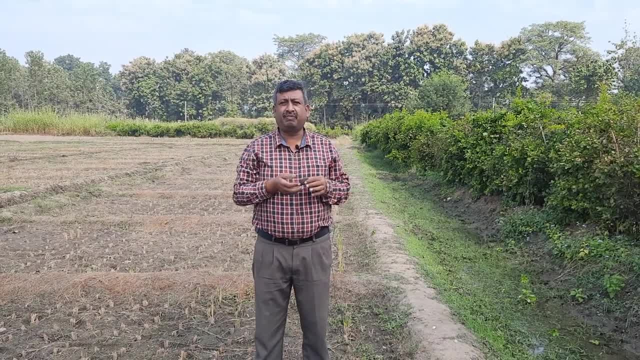 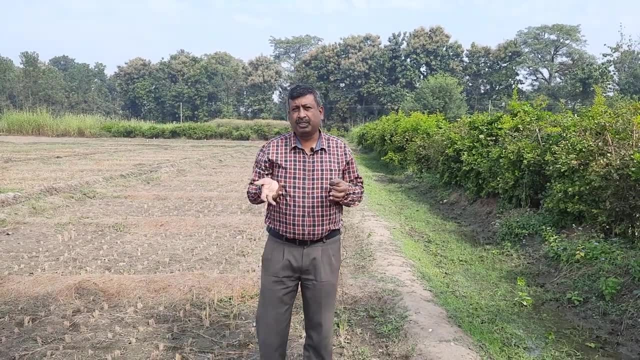 present on this soil is converted into non-exchangeable form. So when it is converted into non-exchangeable form, then when it is converted into non-exchangeable form, the soil will not come into the solution. So another: there is a problem. 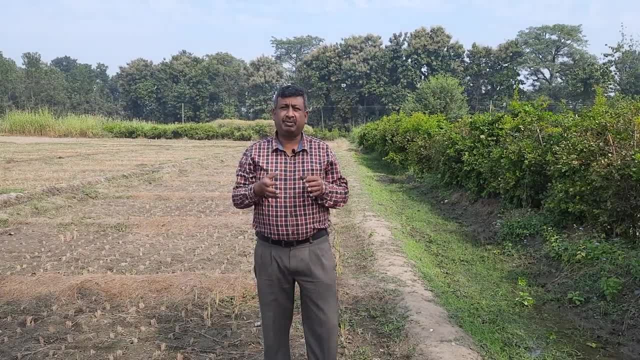 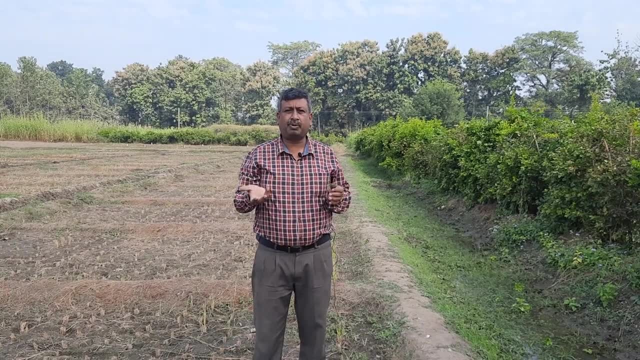 So in acidic condition, In acidic condition and basic condition, alkaline condition- potassium is not available to plant and the best pH for potassium availability is neutral. Neither it is leaching nor it is converted into a non-exchangeable compound. Now another nutrient are calcium and magnesium. behavior is same. 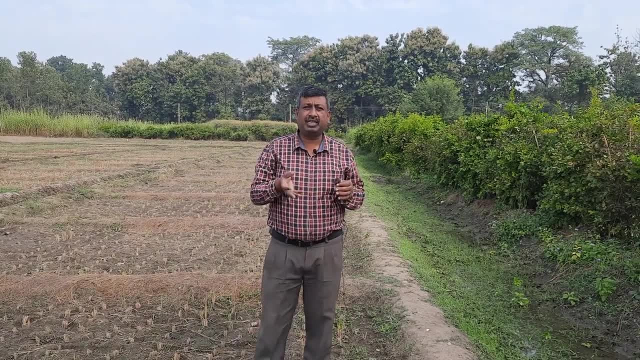 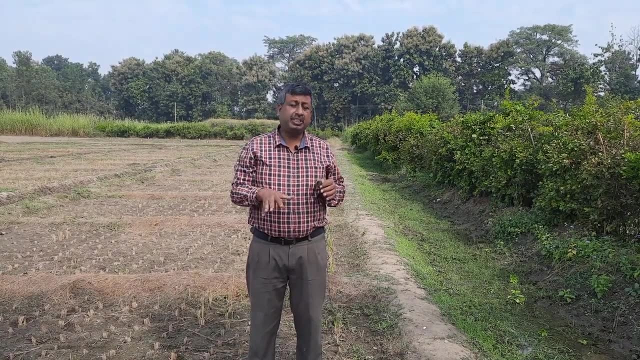 And in acidic condition, same with the potassium. as in the case of potassium, hydrogen dominance is there and hydrogen replaces calcium and magnesium and there is a leaching of calcium and magnesium in the acidic soil. So when leaching will happen, then the soil will not remain in the solution, it will go. 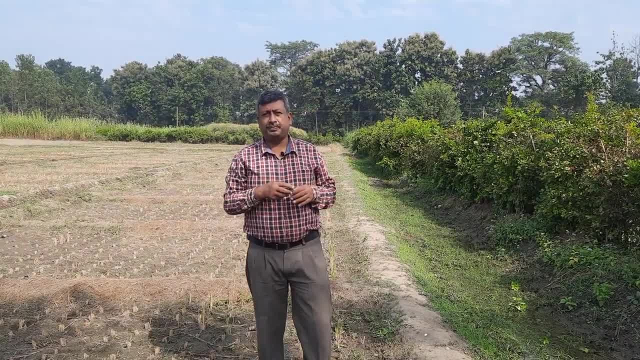 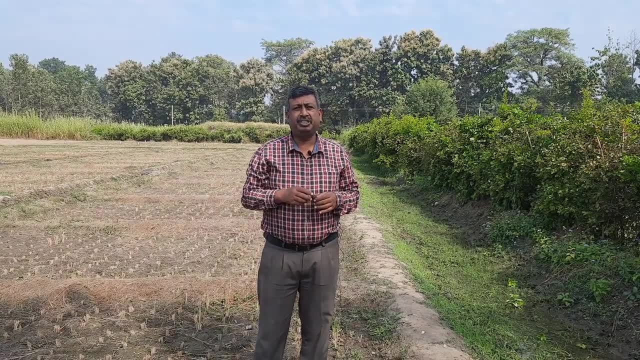 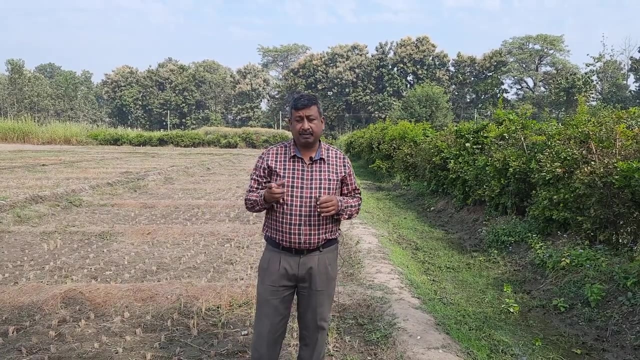 down. That is why calcium and magnesium availability is reduced, And this calcium and magnesium are available at high pH more than 7. So this is a little high range availability when the pH will be more than 7.. Then another nutrient is sulfur. 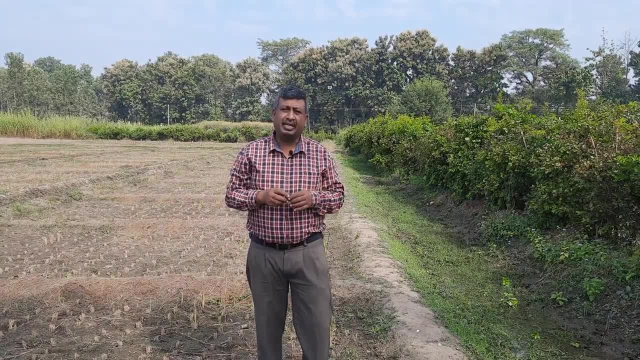 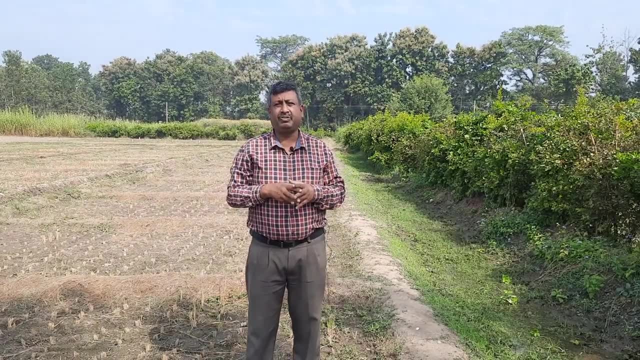 Sulfur behavior in terms of nutrient ability is same as that of nitrogen, because most of the sulfur is present in organic form and available through mineralization and by activity of bacteria, And particularly sulfur oxidizing bacteria. there are a number of bacteria which are involved. 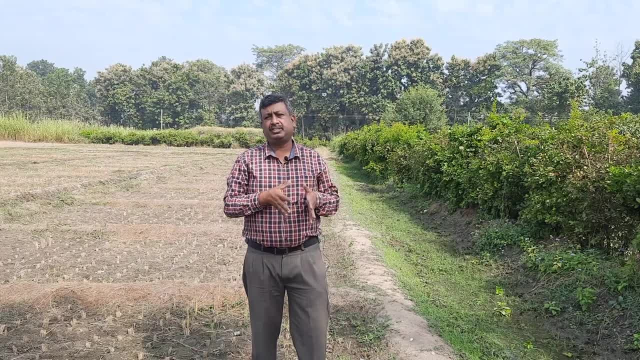 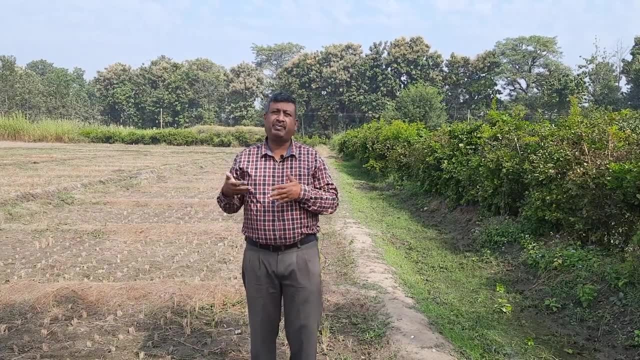 in mineralization of sulfur. So the behavior of sulfur is same as that of nitrogen: when there is organic matter decomposition it will be converted into organic form and it will be available through bacteria. And bacteria perform well at neutral pH. So that is why sulfur availability, again, is maximum at neutral pH. 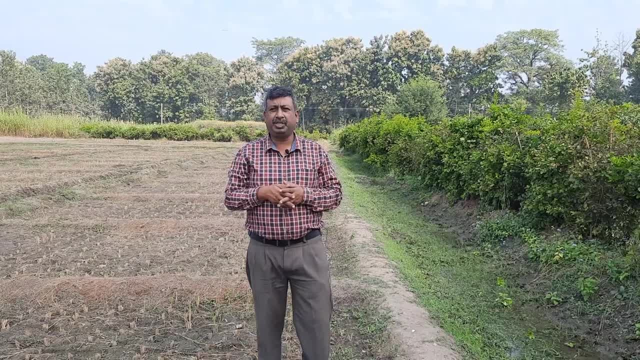 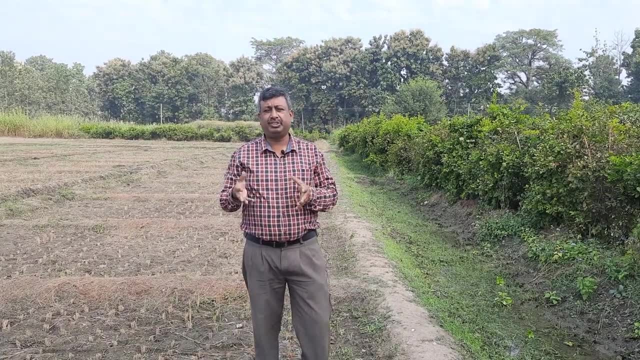 So we have seen this major nutrient: N, P, K, calcium, magnesium, sulfur. So we have seen this macro nutrient. Now we talk about nitrogen. Now we talk about nitrogen. Now we talk about the micro nutrient: Fe, Cu, Mn, Zn, boron, molybdenum. 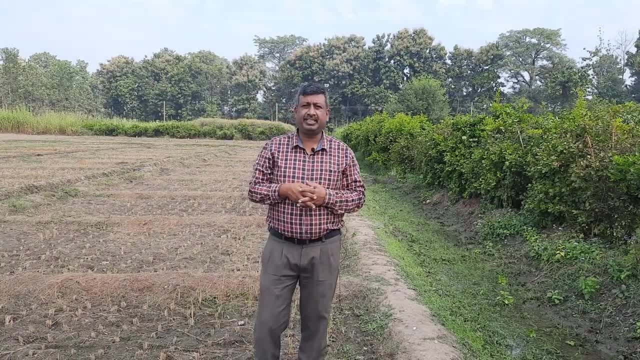 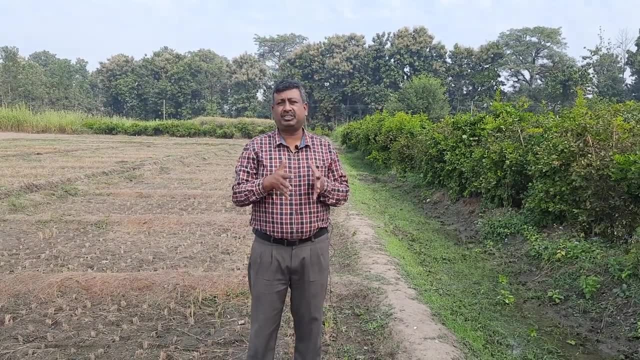 So in this also see the metallic cations Fe, Cu, Mn, Zn. And these metallic cations are more available at acidic pH. When pH is less than 7, about 5 to 6, then availability is very high because solubility. they are soluble at low pH under acidic condition. So that is why under acidic condition there is more availability of iron And sometimes the availability of iron is so high that it shows toxicity. But at high pH these metallic cations are converted into oxide form and hydroxide form. 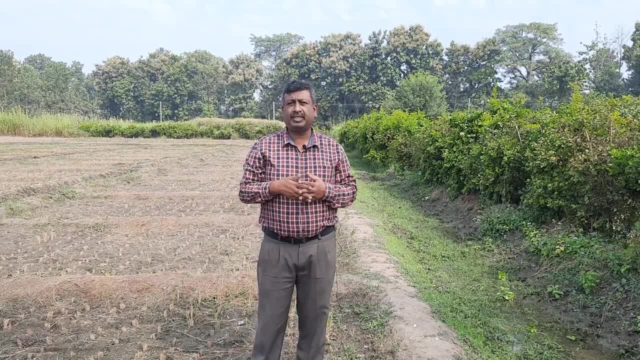 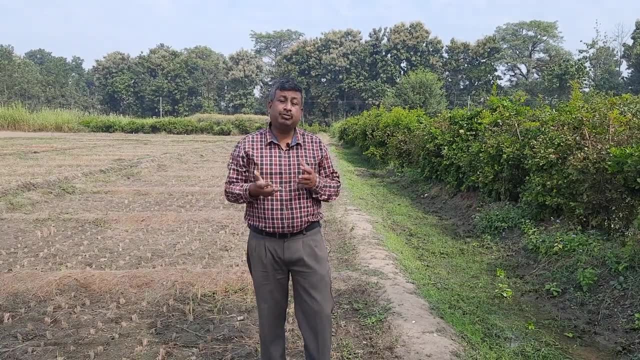 So the hydroxide forms convert on high pH and as the hydroxyl ion increases they react with the hydroxyl ion and they make the hydroxide. And these hydroxides are insoluble. So that is why at high pH these Fe, Cu, Mn, Zn, iron, copper, manganese and zinc are not available at high pH. So these four metallic cations that I have shown you where they can be available, They can be available in acidic range And as pH increases, their toxicity increases and also their acidity increases, So they can be used in acidic range. So these four metallic cations, they are not available at high pH, But at high pH, As the pH increases their availability decreases. so there is a lot of acidity in the soil and it can show toxicity, particularly with iron. so iron will make FeOH whole thrice or FeOH whole thrice, ferrous will make FeOH whole thrice and ferric will make FeOH whole thrice. Zinc reacts with many compounds: Zinc carbonate, Zinc oxide, Zinc hydroxide and many compounds are formed in this. Zinc reacts with SiO4, Zn2SiO4 is formed, then ZnFU2O4,. many compounds are formed in Zinc and Zinc availability is reduced at high pH, so mainly hydroxide is formed. 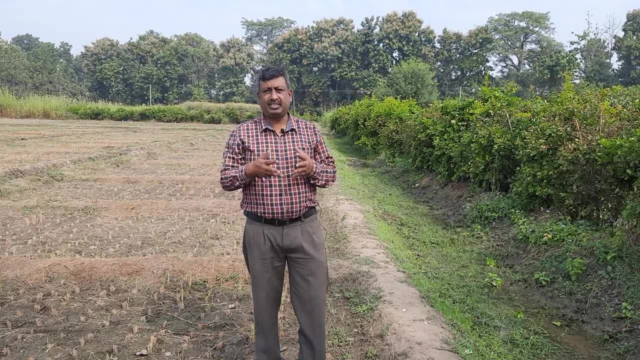 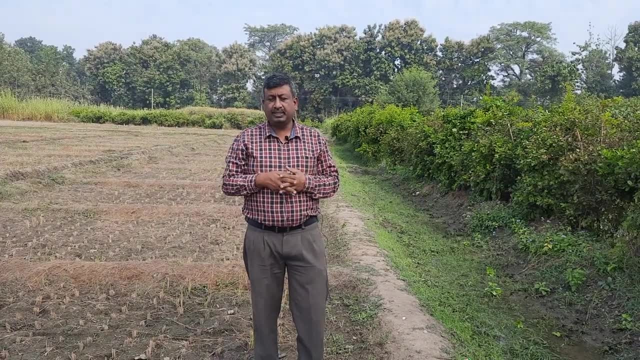 Similarly, in case of copper, CuOH whole, twice copper hydroxide is formed and these hydroxide- copper hydroxide- are insoluble and not available to plant. And in case of manganese, the chemistry is slightly different from Fe, Cu, Ma, Zn. 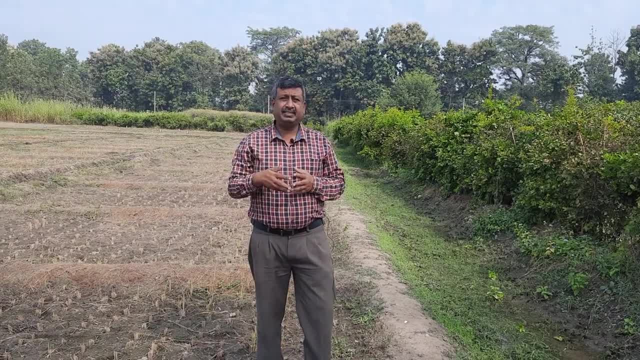 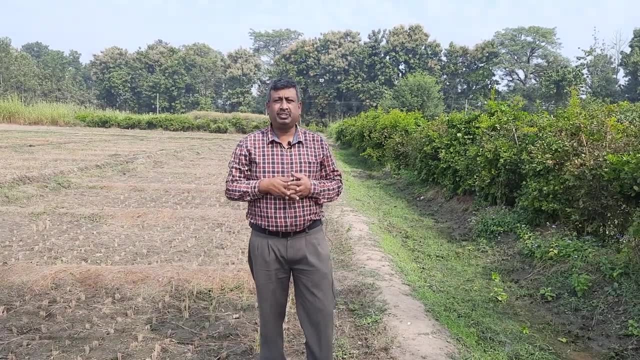 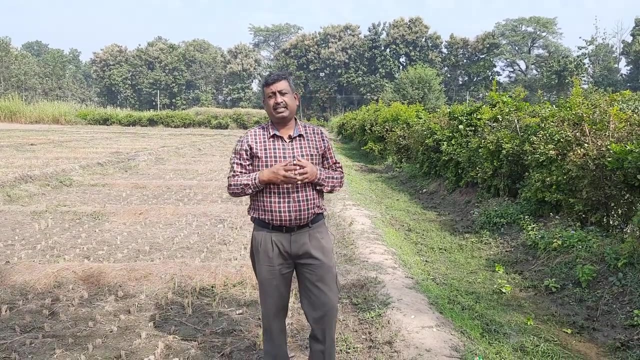 In case of manganese, manganese at high pH is converted into MnO2, manganese dioxide is converted into it and this MnO2 is not available to plant. And another mechanism with the manganese is that it react or make the complex with the organic matter. 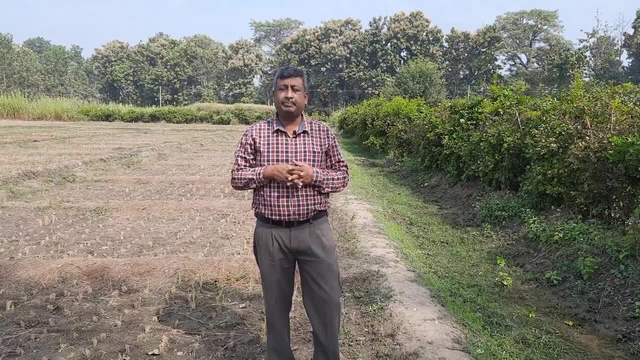 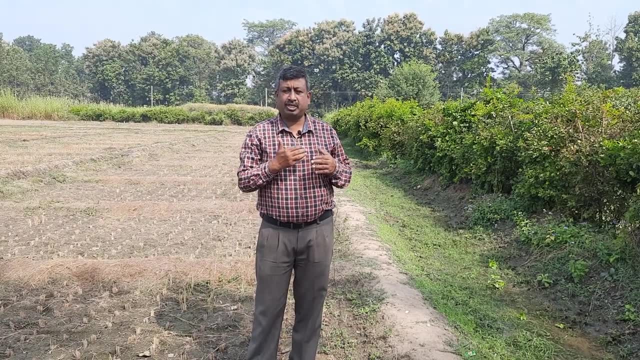 With manganese, there is a reaction. This is the property that it makes complexes with the organic matter, And these organic matter complexes with the manganese are less soluble at high pH. So the organic complexes made in acidic pH are soluble with manganese, But in high pH the organic complexes of manganese are less soluble. 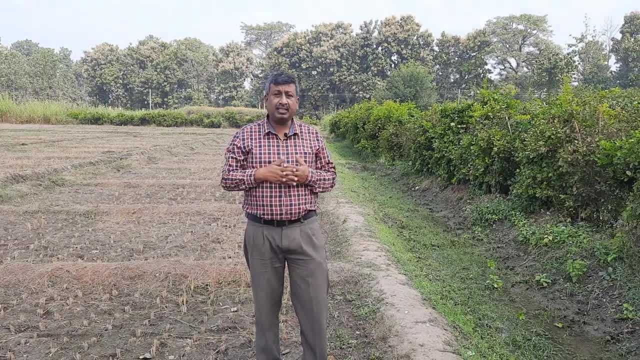 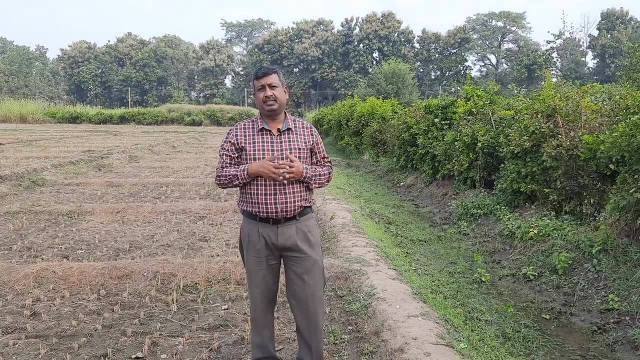 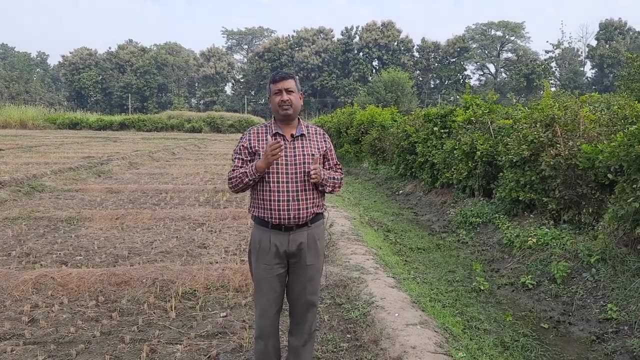 That's why manganese availability is reduced. Then another: this manganese under acidic condition is in divalent form, that is, Mn++, And at high pH it is converted into Mn++ tetravalent form. Tetravalent catain is converted because the bacteria which convert this Mn++ form to Mn++ form are maximum at neutral pH. So as soon as pH goes towards alkaline pH from acidic condition, bacteria population increases and these oxidize the manganese and this manganese divalent form is converted into tetravalent form. And what will happen with that When there is tetravalent form? this tetravalent form is also not available to the plant. 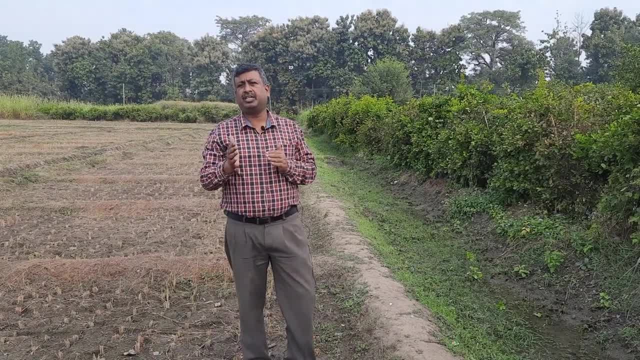 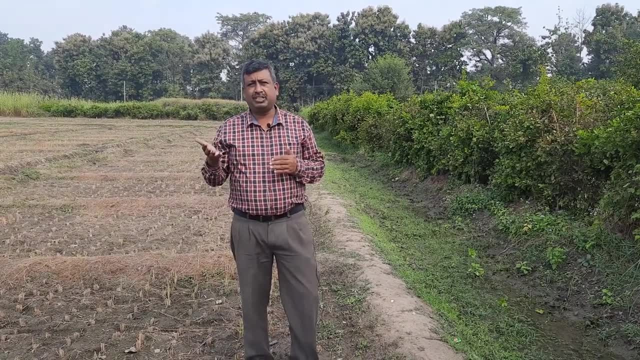 So here we have seen three cases with manganese. One is at high pH. At high pH, manganese is converted into MnO2.. Second, there is more formation of less soluble manganese organic complexes. And third, one is more tetravalent form. 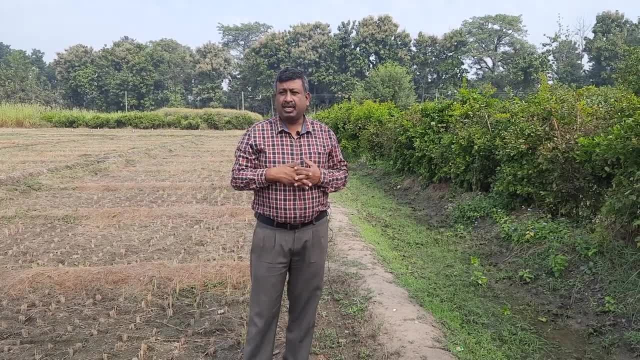 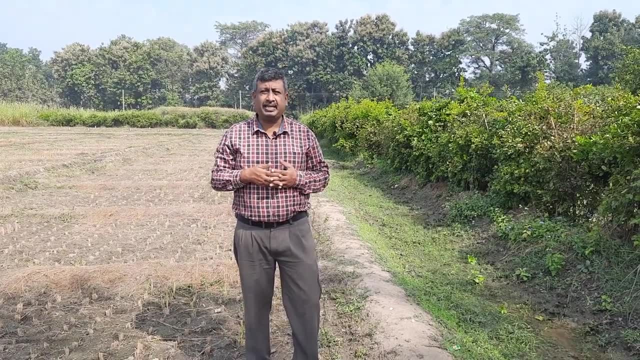 So this is the problem with metallic catain, And there is one more problem with Fe, Cu, Mn, Se, Iron, Copper, Zinc At high pH. they are tightly absorbed At clay, complex organic matter and aluminium and iron oxides. 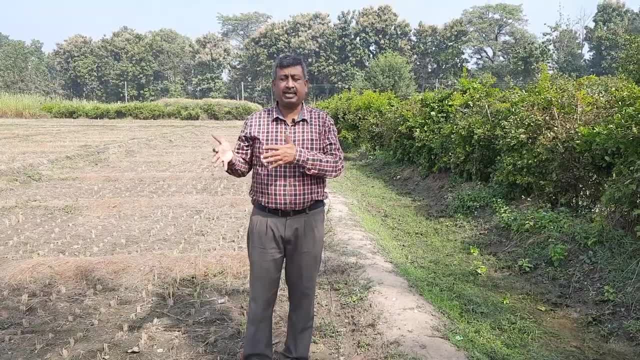 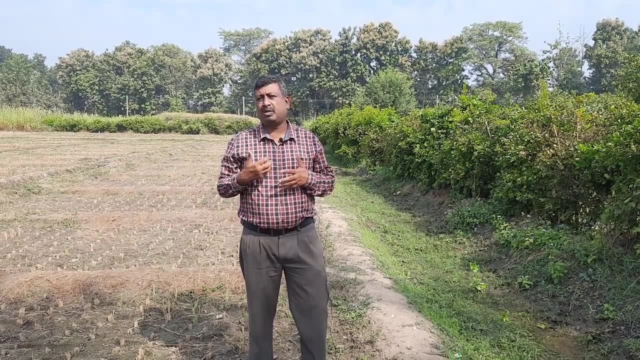 So whatever is in clay or organic matter or oxides or organic matter or oxides of aluminium, iron along with these, they get tightly adsorbed. so when they get tightly adsorbed they will not come in the soil solution, and when they don't come they will not be available to the plant. so this is another problem. 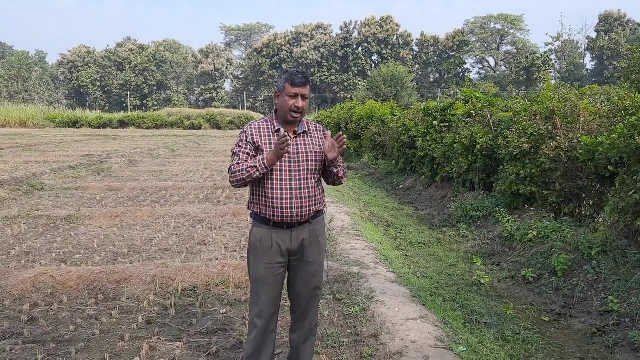 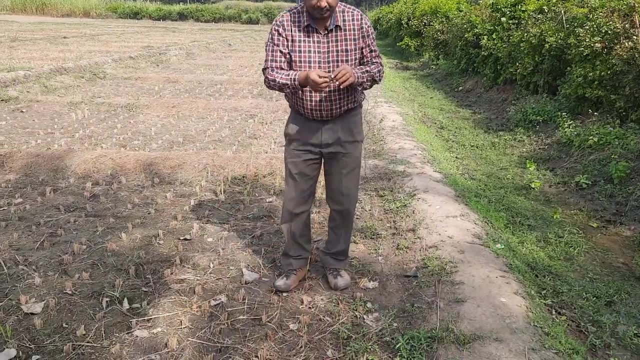 so, first, these metallic cations are converted into hydroxide form, which are insoluble. secondly, they are tightly adsorbed. see the clay complex here. the organic matter or the clay complex in it will get tightly adsorbed. on this, their bonding strength will be very high. 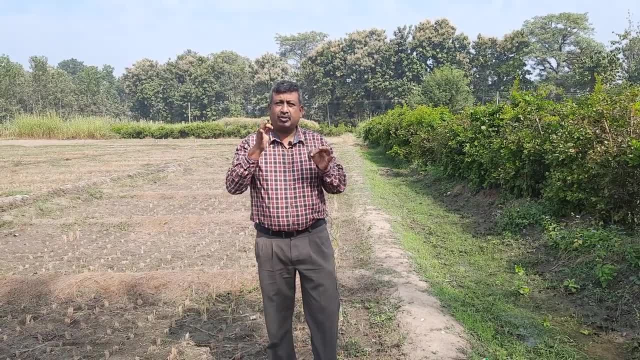 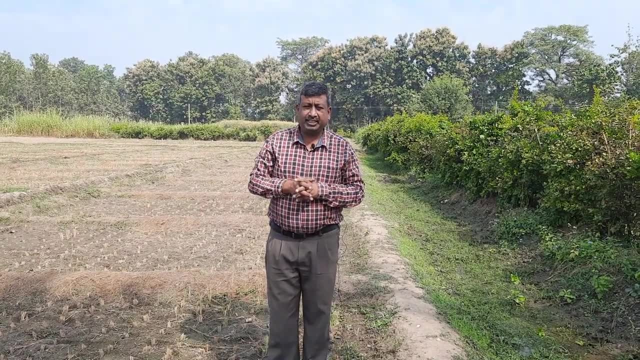 on high pH and then they will not come out of here and will not come in the soil solution, so their availability will be reduced. so this I have just told you about Fe, Cu, M and Zn. if we talk about molybdenum, molybdenum- 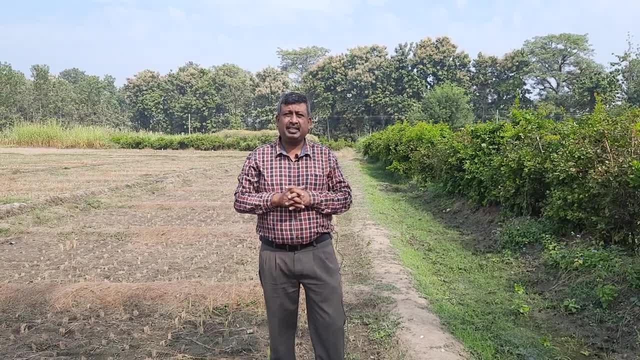 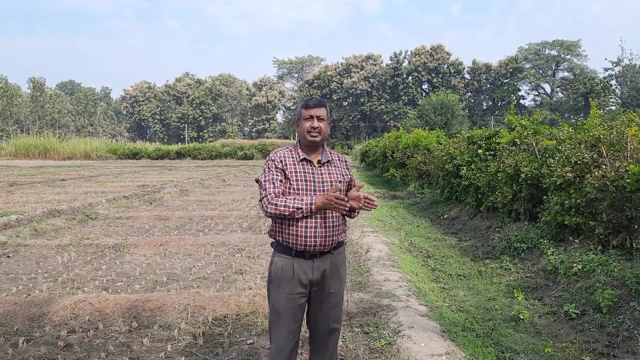 see, it is another nutrient, a micronutrient, but its availability is high, at high pH. so keep this in mind. see, the metallic cations, most of them, except molybdenum, are available at acidic pH, but molybdenum is an exception. it is available at high pH. because it, its available form is MoO4, Divalent anion. it is in anionic form and anionic form is made at high pH. so as soon as pH goes to acidic range it reacts with the hydrogen ion and HMoO4 will be formed, or H2Mo4. 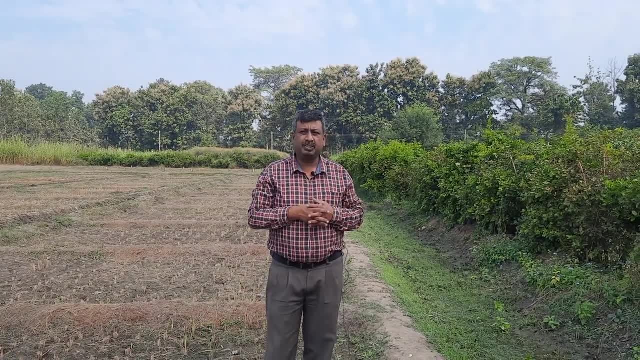 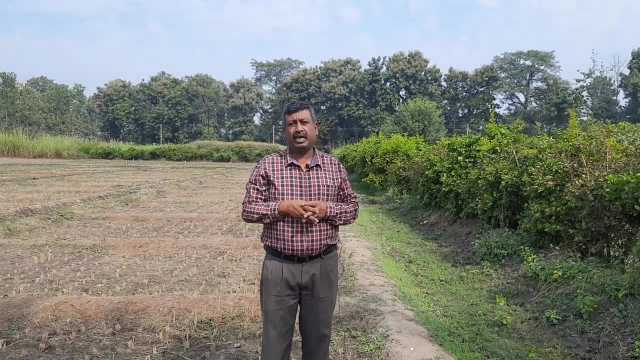 will be formed and when these reaction species are made with hydrogen and these species are not available to plant. so this is the reason that molybdenum is available at high pH. so now we have seen Fe, Cu, M and Zn are in acidic range and molybdenum at slightly alkaline range. the reason for this problem is fe cu, m and gn are in cation form and molybdenum is in anion form, and where shall be anion form to form? it is in high pH. this was the case with molybdenum. 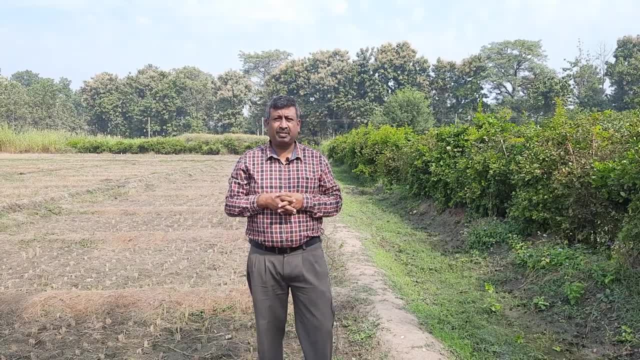 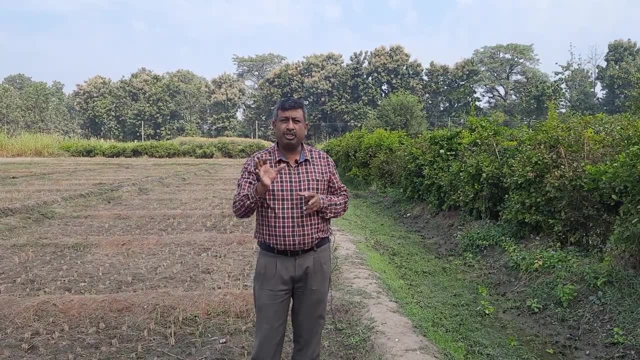 and in the case of boron, boron is generally absorbed in the form of boric acid, CO4, lac than HO3. this is an undisasciated form. dancing here the other form of B4-O7, b4-O7, is also available in this form. 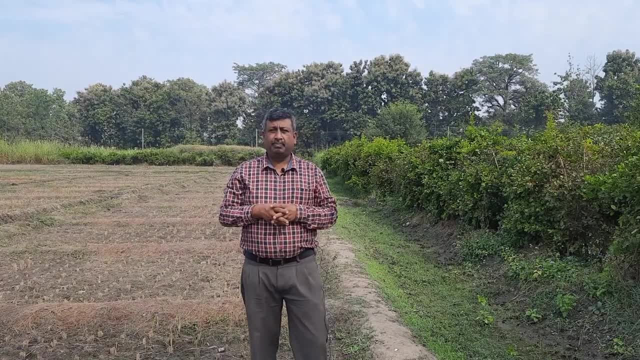 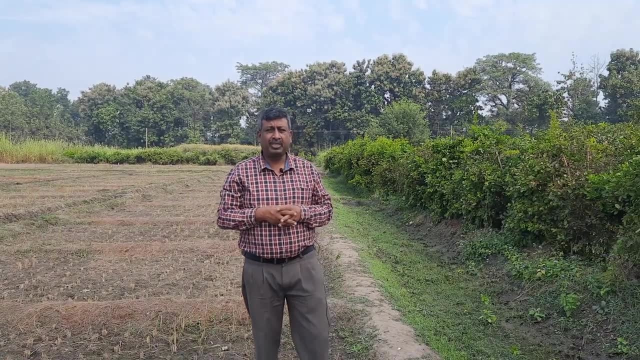 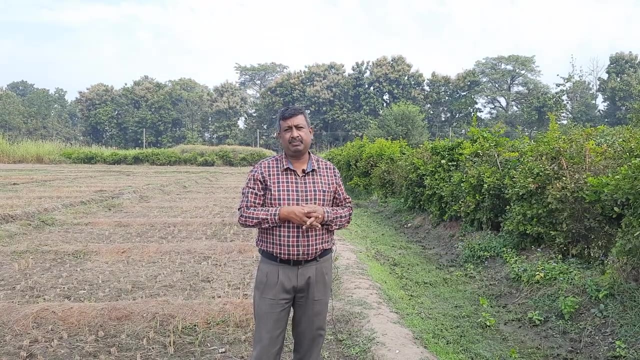 And H2BO4, HBO4 also available, but this solubility is not very good. so boron is in mainly acidic form and see boric acid is H3BO3. definitely its availability will be in acidic range. so this is the reason that boron is available at acidic pH. And as soon as pH increases it will react with hydroxyl ion and it makes H4BO4-, and this anion form is not available, So we can write H4BO4- in BOH4 and H4BO4- as well. 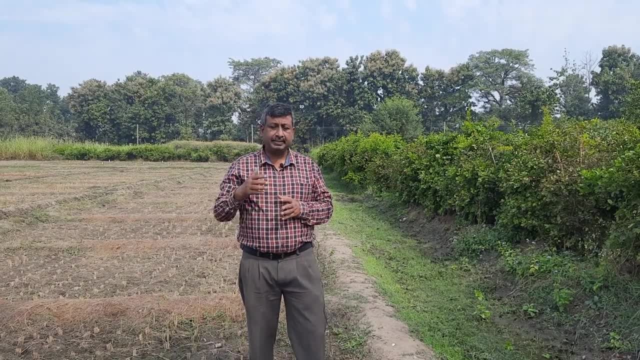 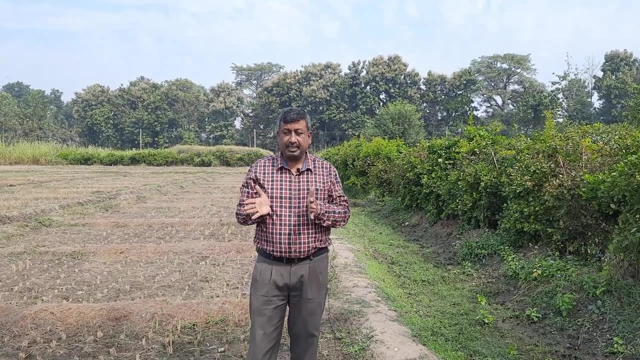 And this form H4BO4- is made at high pH only, And this form, H4BO4- is made at high pH only Because it is not available. that is why boron availability is reduced And we can see that boron availability is in acidic pH only. 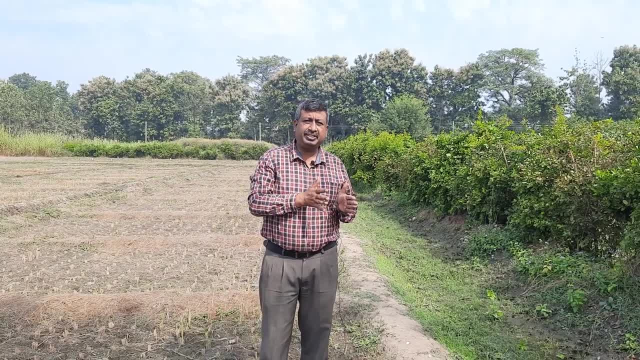 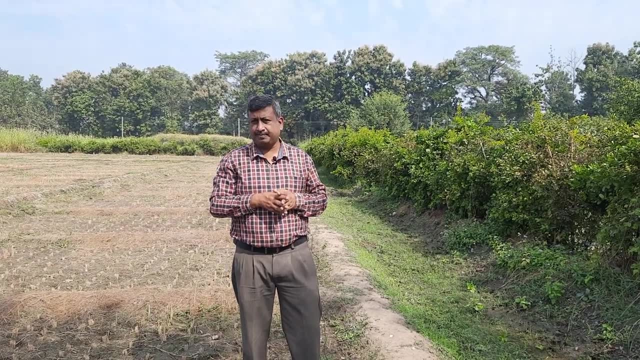 That is why boron is available at high pH, So we can see that the micro nutrients are in acidic range And molybdenum is in high range, And because the requirement of micro nutrients is very less. So if it will be very available, then it shows toxicity. 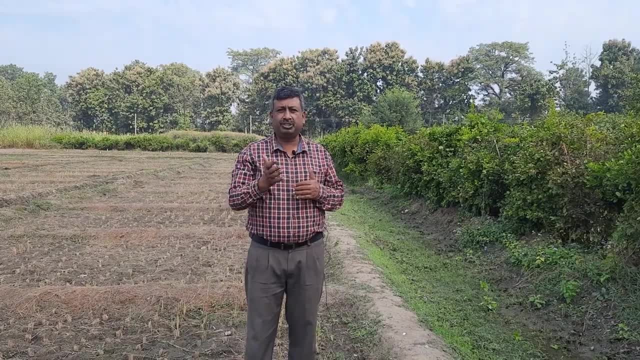 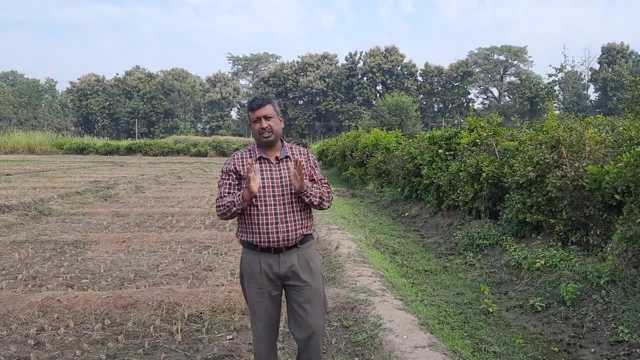 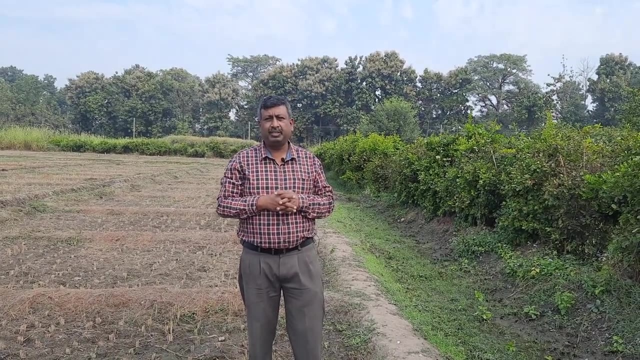 So we don't have to make the availability very high, otherwise there can be toxicity. So the neutral pH is very good from the nutrient availability point of view. So we have seen how nutrient availability is affected by pH. So most of the nutrients are maximum at neutral pH 7.. 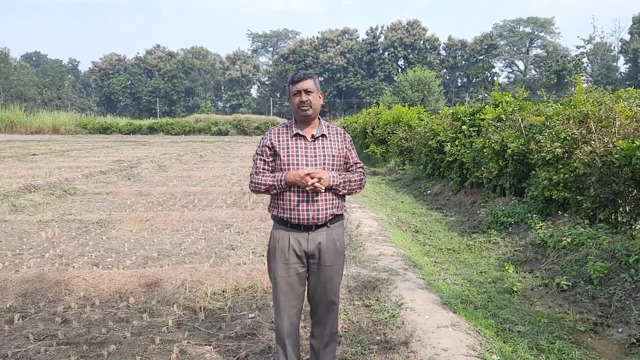 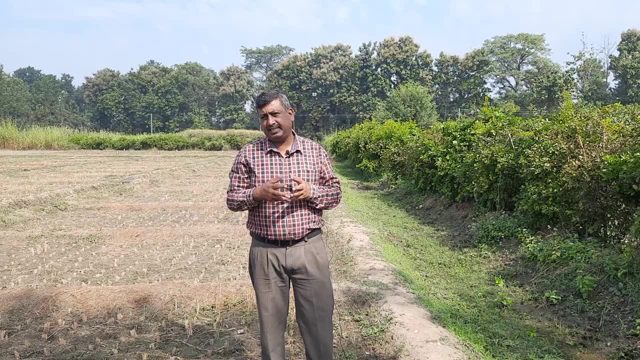 So if the neutral pH is of soil, then nutrient availability will be more. So this was the effect of nutrient availability And how did it show It was affected by solubility. So this was the first factor that I told you. 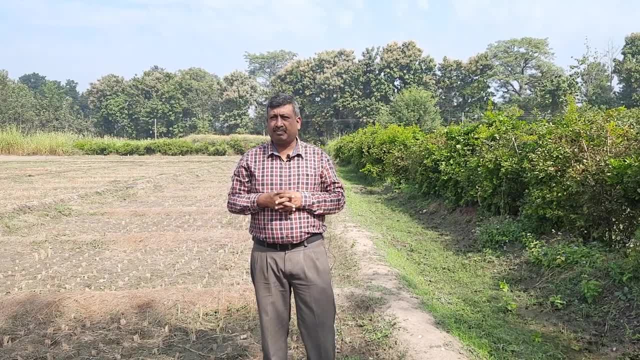 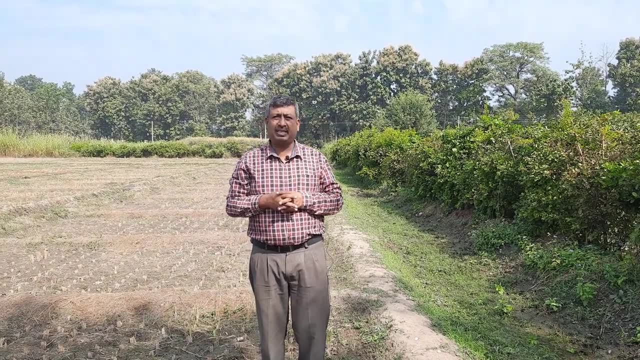 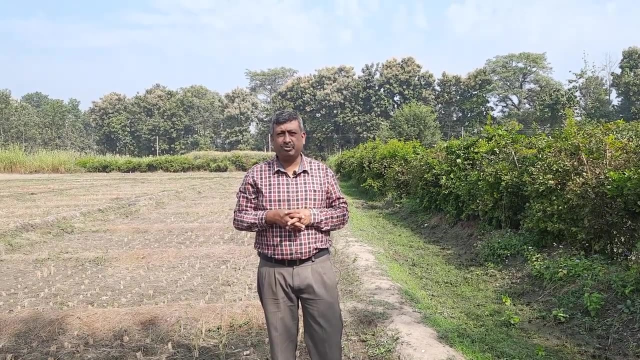 And the second factor is microbial activity, And microbes are involved in decomposition And we had just discussed, as in case of nitrogen and sulphur and manganese. So see where the microbial activity is maximum, at neutral pH. That's why nutrient availability will be very high at neutral pH. 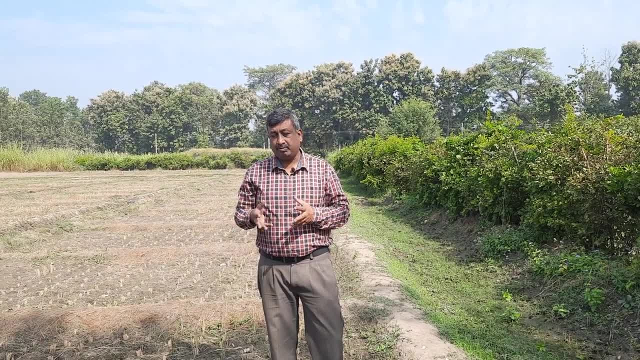 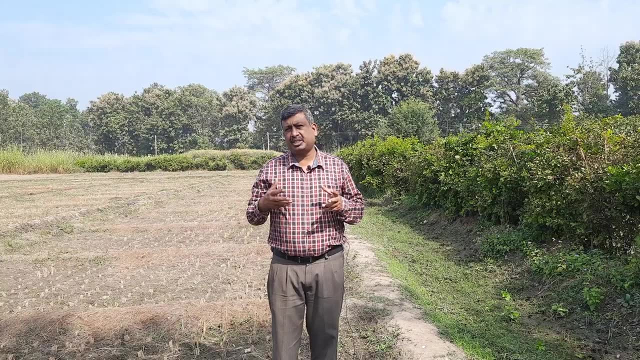 So here the microbial activity, particularly bacteria, is involved in decomposition. So the mineralization rate will be the highest at neutral pH. So the second factor is where our maximum is at neutral pH, And the third factor is the cation exchange capacity. 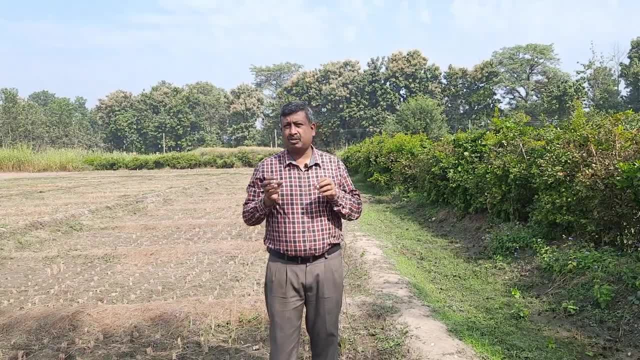 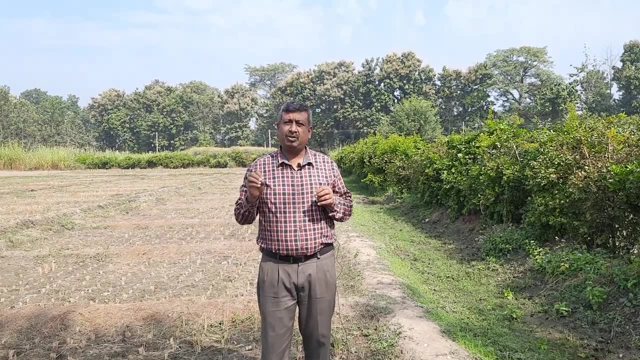 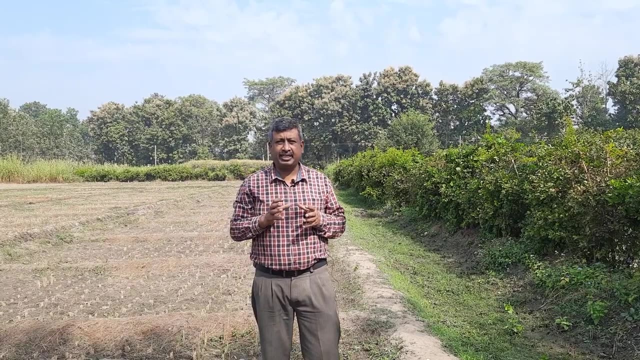 This is a very important factor. I had told you earlier that nutrient should not only be present on clay complex. It should be in exchangeable form and it should be in soil solution. Otherwise it will not be available to plant. So the soil capacity will decide how much nutrient will come in the solution and how much will not come. 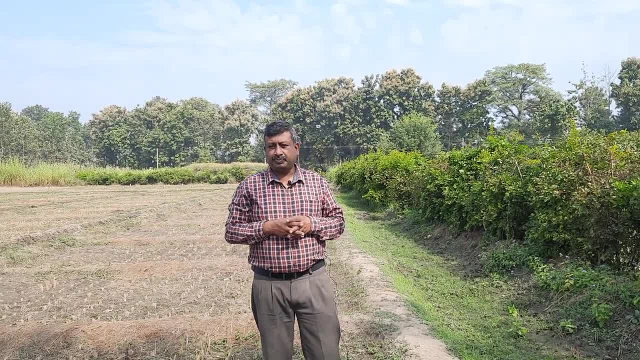 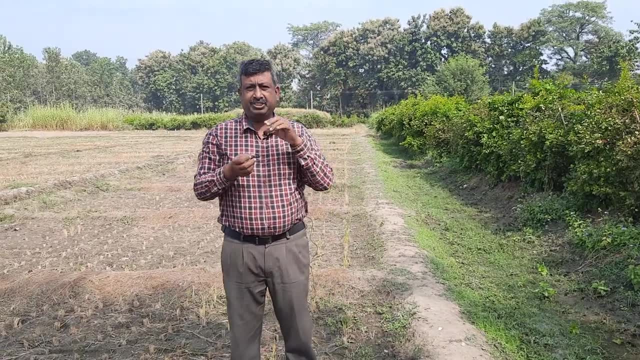 And this capacity is known as cation exchange capacity. Now we will have to understand this cation exchange capacity a little bit. See, this clay particle is soil. It is negatively charged. Now in this negatively charged particles, the negative charge comes by two means. 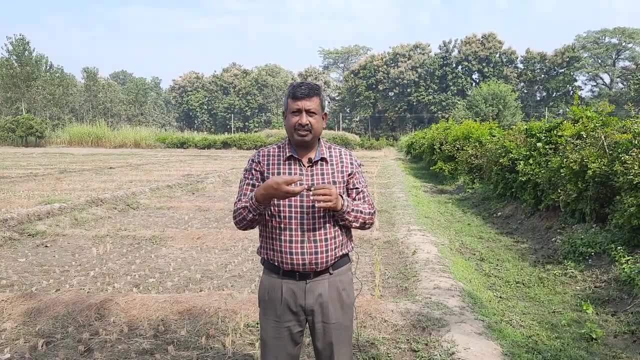 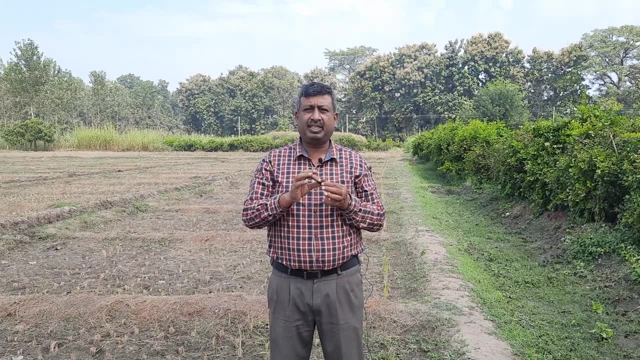 It comes in two ways And this negative charge is kept by holding the cation And it is exchanged with the soil solution. If the negative charge is reduced in this, then the cation holding capacity will be reduced And whatever fertilizer we will give, nutrient will be leached. 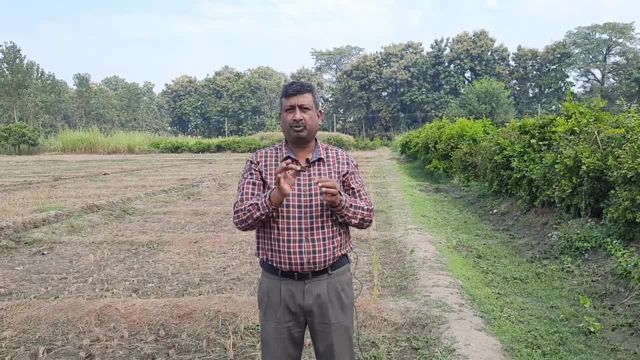 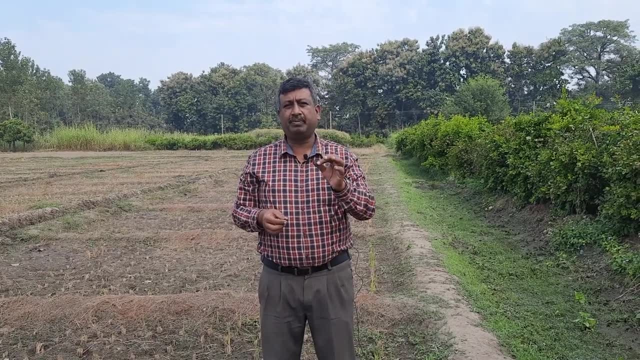 So to prevent leaching. To prevent leaching, it is very important to have its clay complex, And for the plant to be available it needs to have a soil solution. So see, both the phenomena are important. One is in the soil solution and the other is in holding the soil. 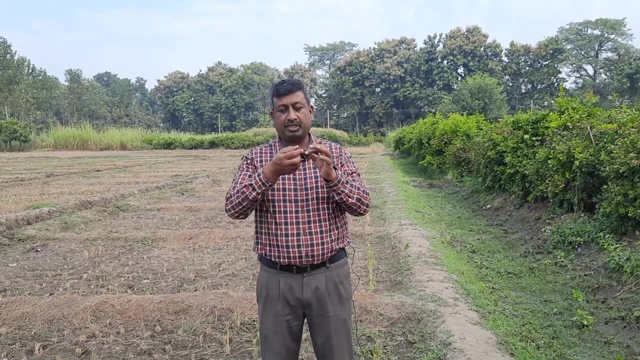 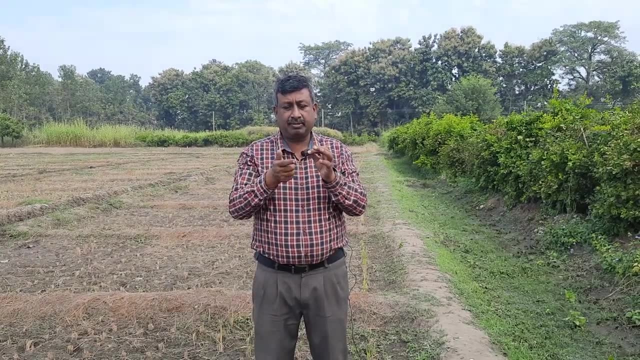 So there should be an equilibrium between the two. If the soil does not hold it at all, then it will leach down and not be able to plant. If the soil holds it tightly and does not exchange the soil solution, then there will be no nutrient in the soil solution and it will not be able to plant. 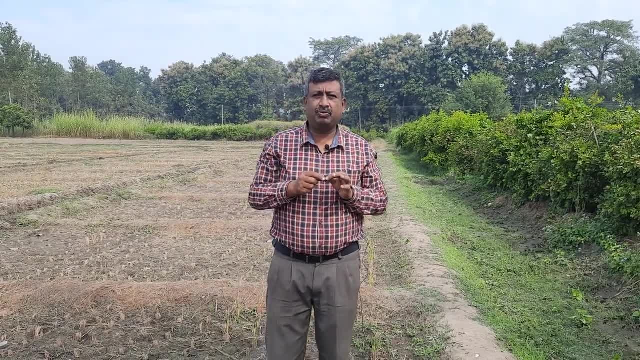 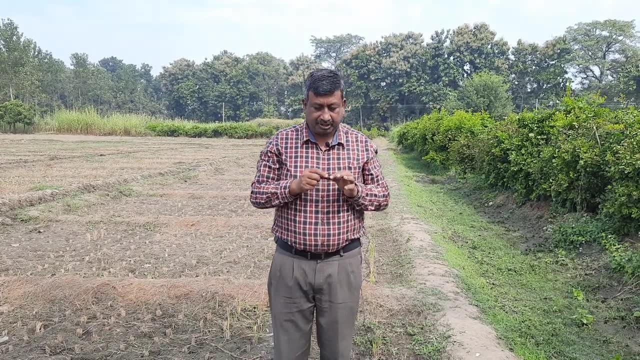 So see both the extreme conditions Here: nutrient will not be available and soil fertility will be poor. So there should be an equilibrium In the holding capacity and in its exchange. So cation exchange capacity is very important. Now these negative charges come in two types. 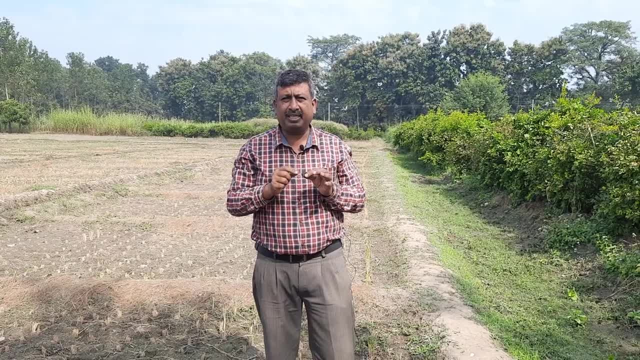 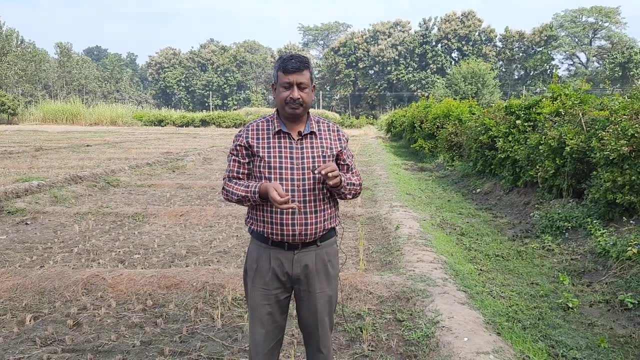 One is permanent charge, Permanent negative charge, which is always present in it, And these permanent charges are due to isomorphic substitution. So isomorphic substitution is a phenomenon, From that permanent charges come. Second is some carboxylic group and phenolic groups are present. 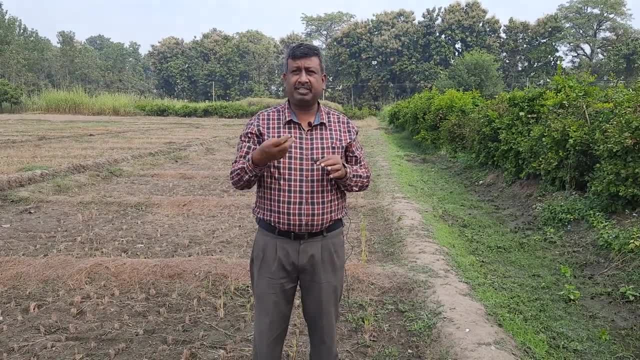 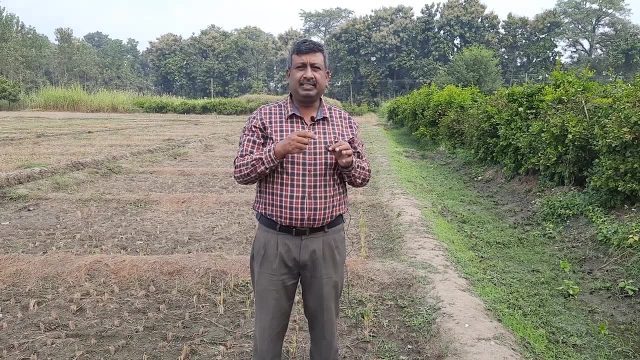 And this carboxylic group and the group that comes from the organometer and acids. What are they? They are pH dependent charges Under acidic condition. these phenolic and carboxylic groups are less Because the dominance of hydrogen reacts with them. And as the pH is increased, these carboxylic, phenolic and other negative charges increases, And this type of charges are known as pH dependent charges. So see, there are two types of charges: Permanent charges and pH dependent charges. So their sum will be total negative charges And those total negative charges will hold all the cations and exchange them. So we will have to see Where will the permanent charges and pH dependent charges be the maximum. So see, the pH of the permanent charges will not be affected. The pH will not affect it, Whether it is acidic, alkaline or neutral. the permanent charges will remain the same, But the pH dependent charges. these charges are minimum in acidic condition Because the hydrogen blocks them by reacting with them. So the pH dependent charges will be less in acidic condition. 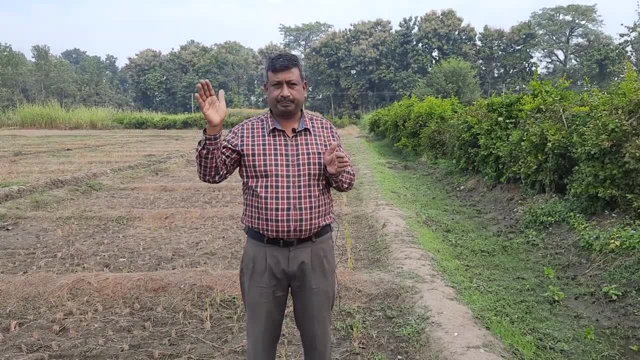 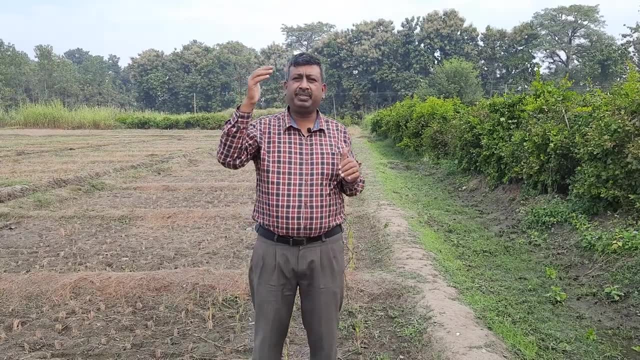 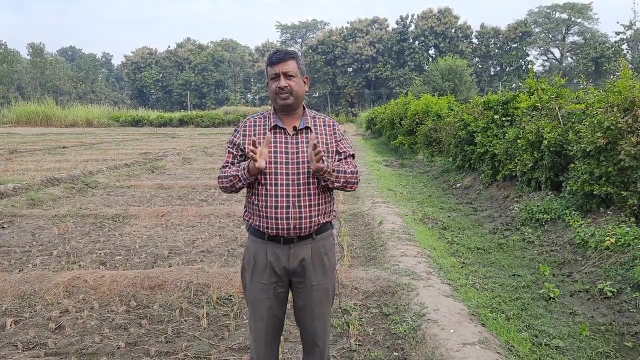 As the pH is raised, these pH dependent charges increase And these pH dependent charges become maximum by reaching pH 8.. So this means that if our pH is around 8 or 7, then our total negative charges will be more, And when total negative charges are more, then cation exchange capacity will be more and there will be more nutrient availability. 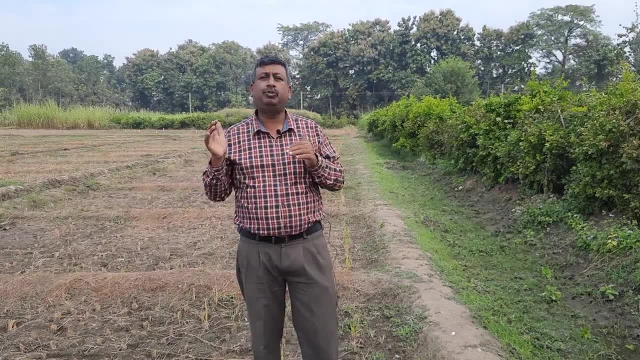 So the CEC in general it is maximum at 7 to 8.2 pH. So see, this also went from a neutral pH to alkaline. So 7 to 8.2 pH in general is maximum. 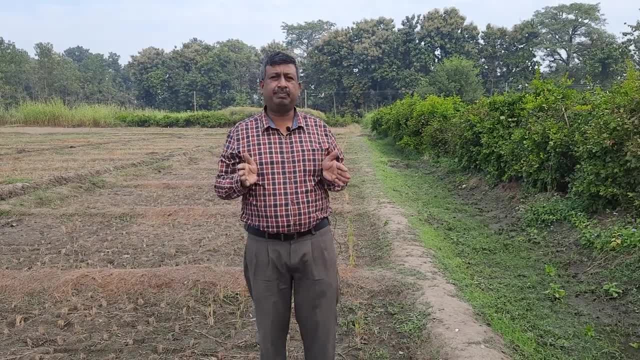 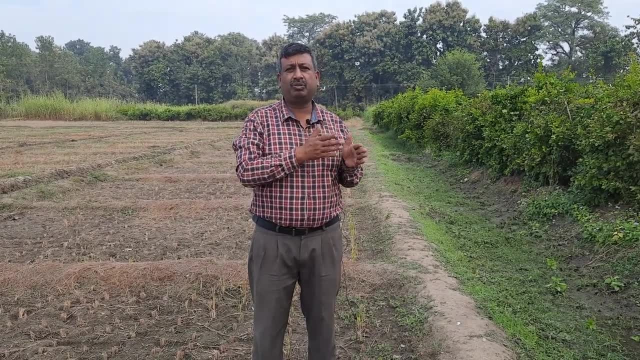 7.2 pH in general is the considered best for maximum cation exchange capacity. So see here, the CEC is also coming in the neutral range. Now we saw nutrient solubility. Most of the nutrients are soluble at neutral pH. 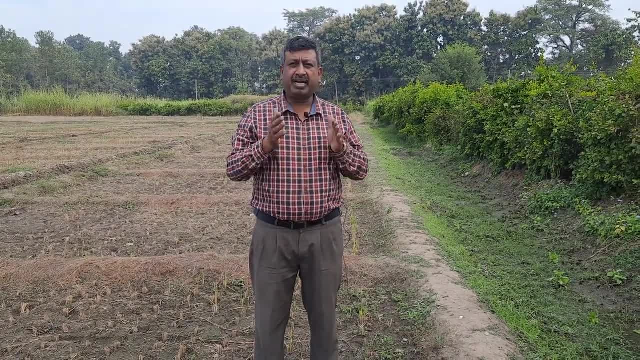 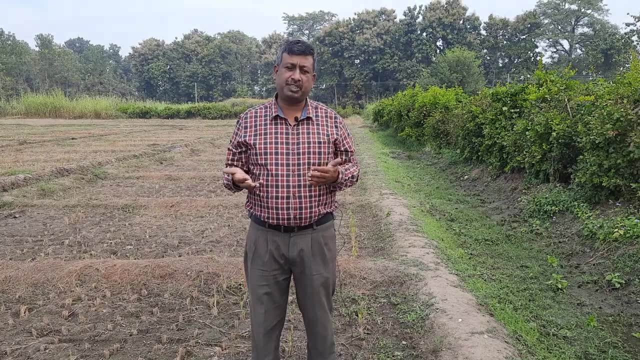 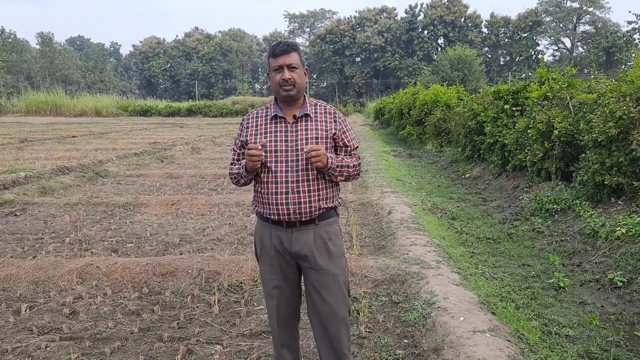 Maximum microactivity is maximum at neutral pH. Maximum CEC is at neutral pH. So what happened is that the maximum nutrient availability will be at neutral pH. So that's why our soil pH should be neutral to get maximum nutrient And by the plant. 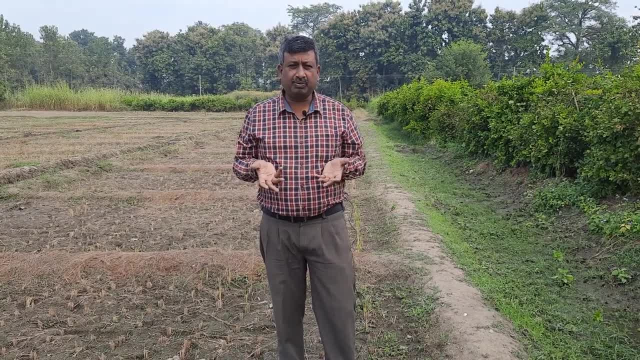 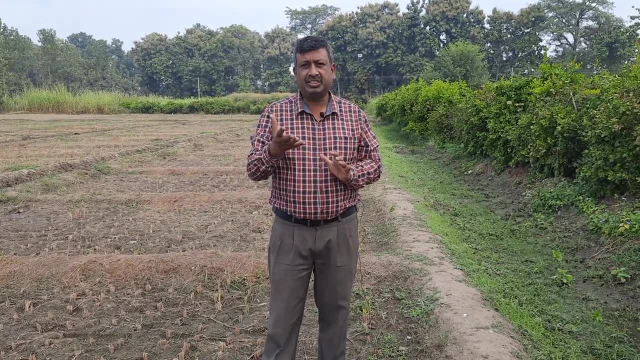 So if this pH is not neutral, then nutrient solubility will be affected and definitely crop performance will be poor. So if there is disturbance in the soil pH, then we reclaim it. So this was today's lecture: to tell you how pH influences nutrient availability. 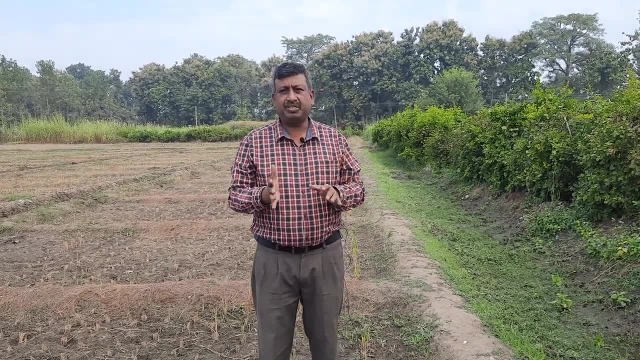 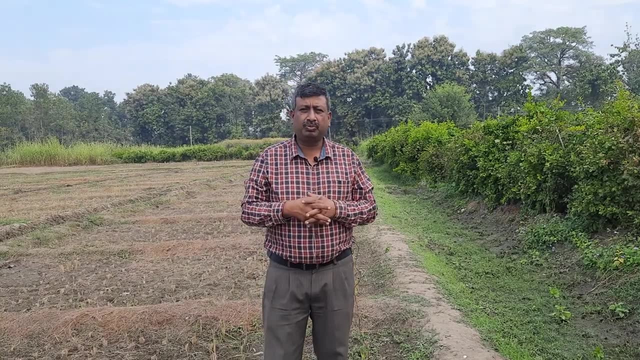 Let me brief you again. This nutrient availability is affected by three means. Number one, nutrient solubility. Second is microactivity. And third one is cation exchange capacity. So I hope you liked this lecture. You must have understood. 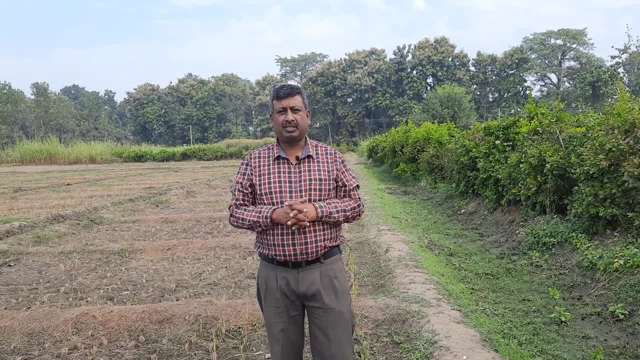 If you liked it, then like it, share it, And if you haven't subscribed to the channel, then subscribe to it. Thank you very much.